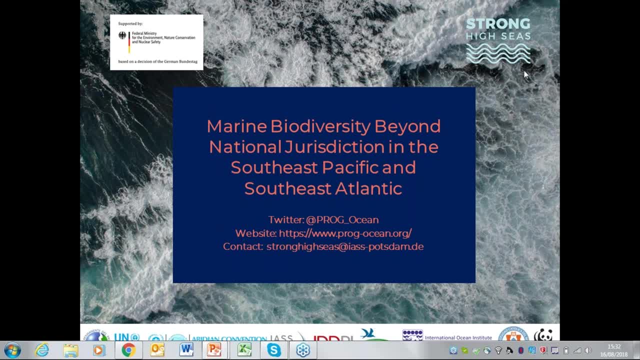 on the 3rd of September and an expert workshop meeting on the 8th of September, also as part of the BB&J negotiations, and in New York. So please get a hold of us if you have interest in attending these events that are going to be in New York. Before we get started, we 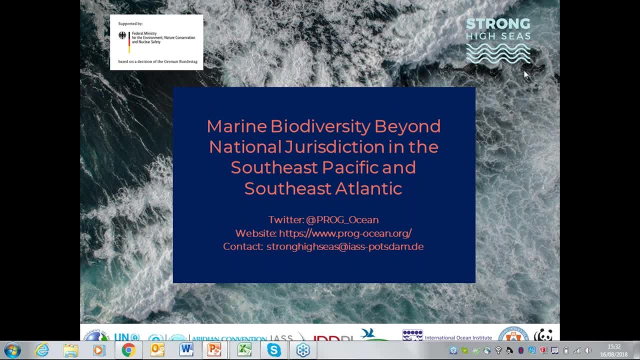 just wanted to take a few minutes and tell you a little bit about the Strong High Seas Project. This is a five-year project. It started in June 2017 and goes until May 2022.. It's funded by the German Federal Ministry for the Environment, Nature Conservation and Nuclear. 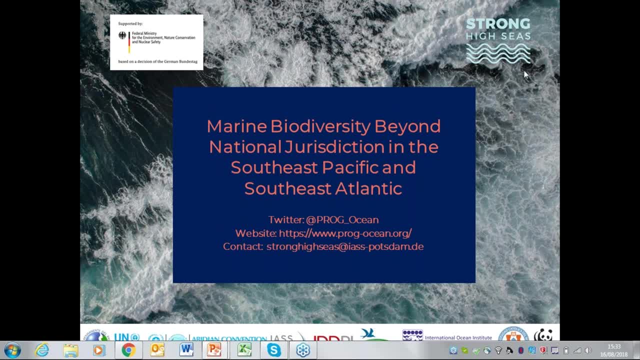 Safety through the International Climate Initiative, so the ICI initiative. It's coordinated by the Institute for Advanced Sustainability Studies and has implementing partners: Institute for Sustainable Development and International Relations in Paris, France, the International Ocean Institute of South Africa, the Universidad Católica del Norte, UCN and WWF Germany. 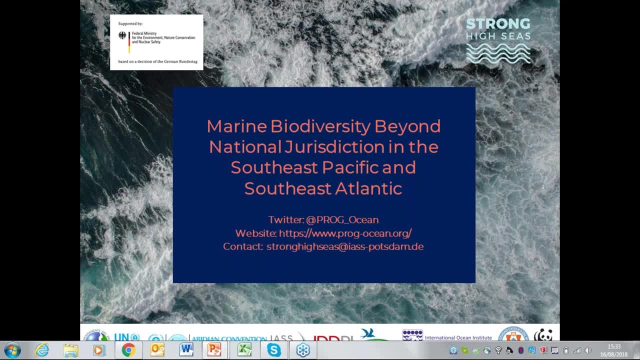 as well as some of the other partners: The Institute for Advanced Sustainability Studies, as well as some of the partners that we have here presenting today, which is BirdLife International Africa and WWF Colombia. We also have the regional partners, who are co-hosts here today's. 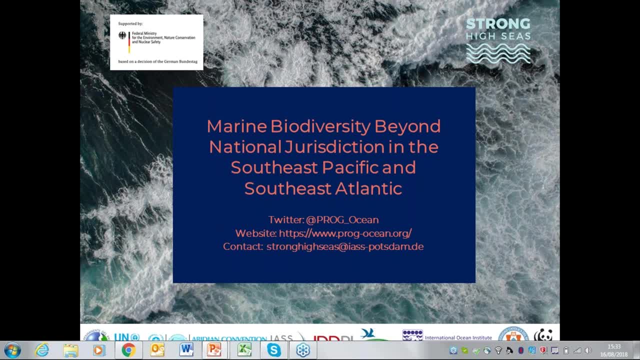 Abidjan Convention Secretariat and the Permanent Commission for the South Pacific. So the objective of the Strong High Seas Project is to develop and support new approaches for ocean governance towards approved conservation and sustainable management of marine biodiversity in areas beyond national jurisdiction. The project works in three primary ways. First, it works within two specific regions. 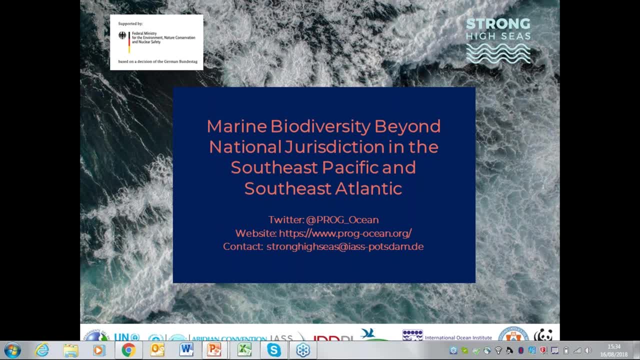 being the southeast Pacific, so the west coast of South America and the southeast Atlantic, the west coast of Africa, and here it tries to engage with local stakeholders, governments, private sector, scientists and civil society to support integrated management approaches for the conservation and sustainable use of biodiversity and then facilitate the delivery. 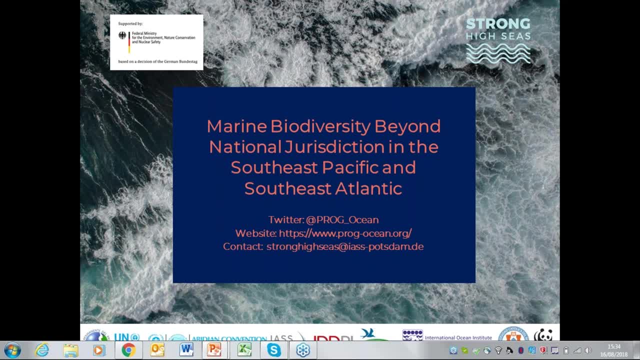 of these proposed approaches into relevant regional policy processes. The second primary way the project works is it focuses on inter-regional exchange between different marine regions regarding best practices and lessons learned for ocean governance, in an effort to support the sharing of knowledge and information. And finally, the project explores links and opportunities for regional governance in a 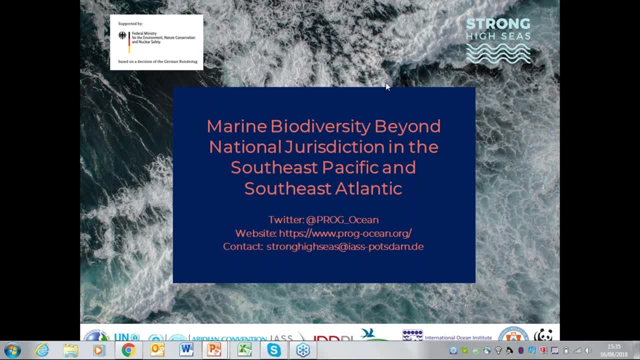 new, internationally and legally binding instrument on marine biodiversity in the high seas, which is currently underway in negotiations in New York next month. So today we have a great webinar planned for you over the next hour. First, we're going to hear from Professor Pat Halpin, along with Professor Daniel Dunn and 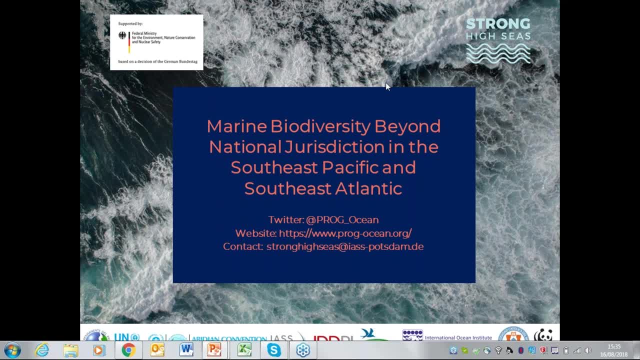 Guillermo Crespo, a PhD candidate, all of Duke University's Marine Geospatial Ecology Lab, About the latest science on the importance of global marine biodiversity in areas beyond national jurisdiction. After the presentation, we're going to have a first Q&A session for about 10 minutes. 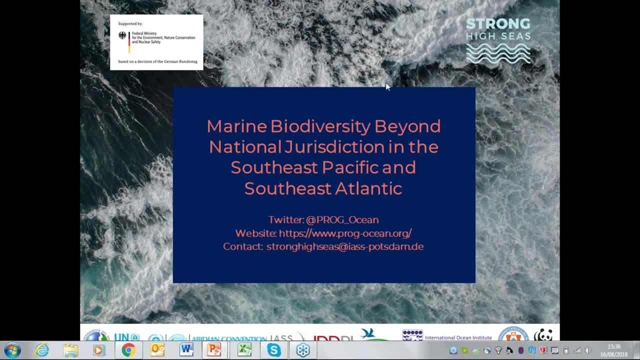 And after that we will have two more presentations where Dr Ross Wanlis from BirdLife International and Johanna Pruessmann from WWF Columbia will provide specific examples of marine biodiversity and challenges faced in areas beyond national jurisdiction In the Southeast Pacific and Southeast Atlantic. 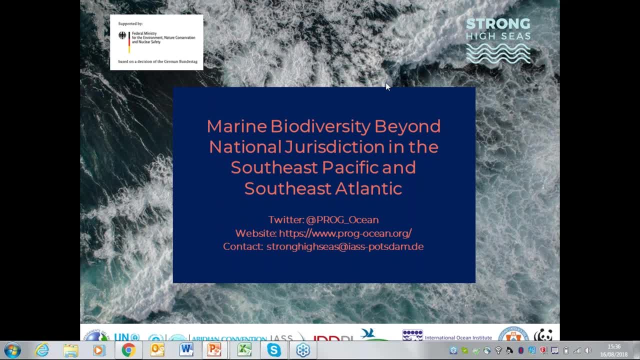 This then will have another Q&A session following these two presentations. So please write your questions into the box on the side, if you have one, and you can write them in during the presentations as well, And we will get to the questions during the Q&A session. 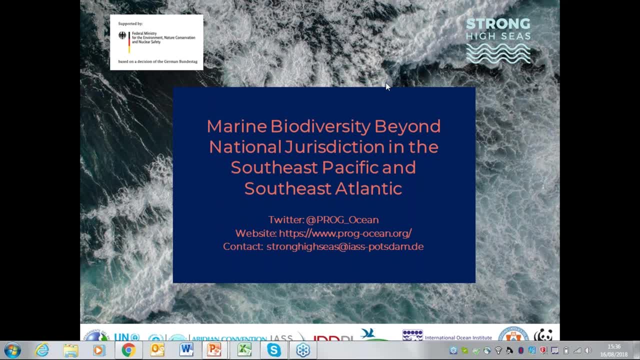 So all microphones of participants have been muted, so you're aware, And also we will be recording the webinar And posting it online afterwards And as well, you should receive a short five-question survey after the webinar. So please take a few moments and fill this out, as this would help us a lot. 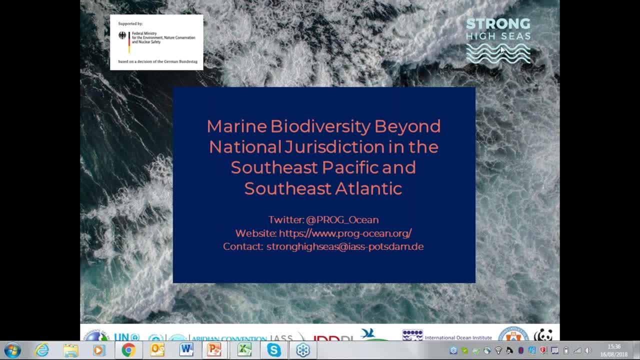 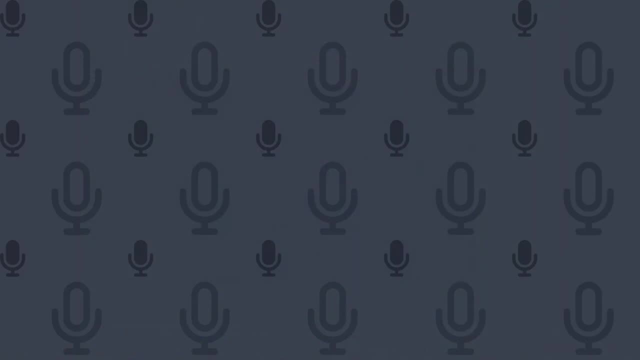 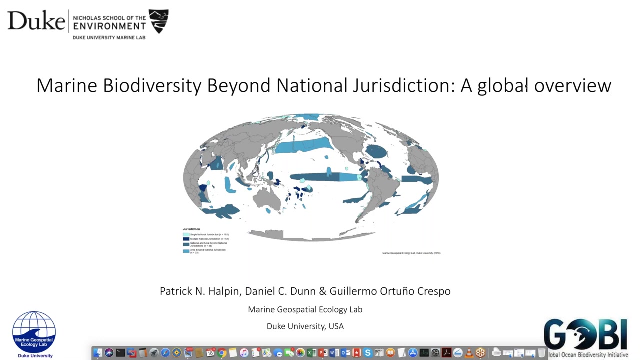 Thank you. Yes, good morning. My name is Pat Halpin. I hope that you can hear me well. I'm from the Marine Geospatial Ecology Lab And I'm going to be presenting on marine biodiversity beyond national jurisdiction, And also my colleagues Daniel Dunn and Guillermo Ortuño-Crespo are here to talk about marine. 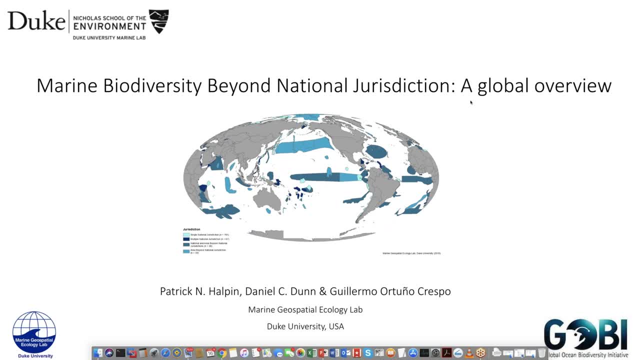 biodiversity beyond national jurisdiction. They're here from Duke University, So this is a very, very broad topic And we have just 10 minutes to go through it, So we're going to be fairly superficial And hopefully we can catch questions at the end if you have particular questions. 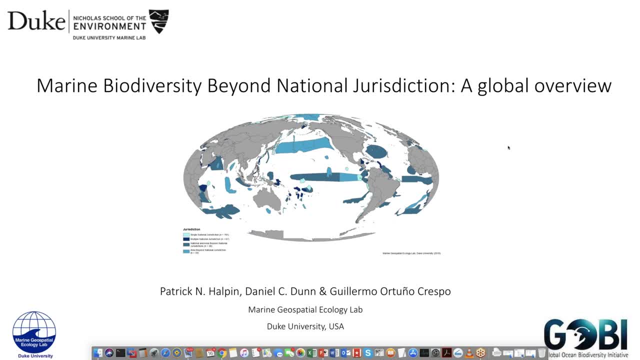 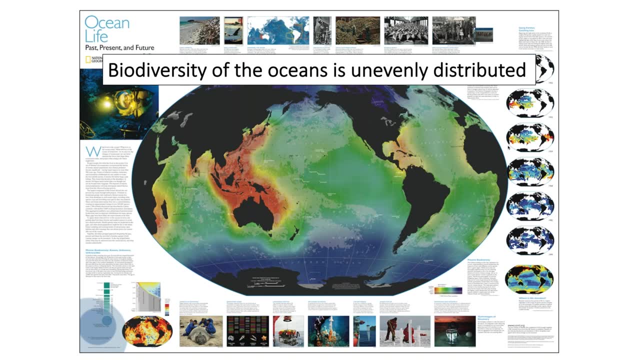 So, to begin with, biodiversity beyond national jurisdiction is really unevenly distributed in the oceans, And this is important because a one-size-fits-all solution to our governance and management of biodiversity is not going to succeed, And so we need information, and detailed information on the biodiversity of the oceans by different 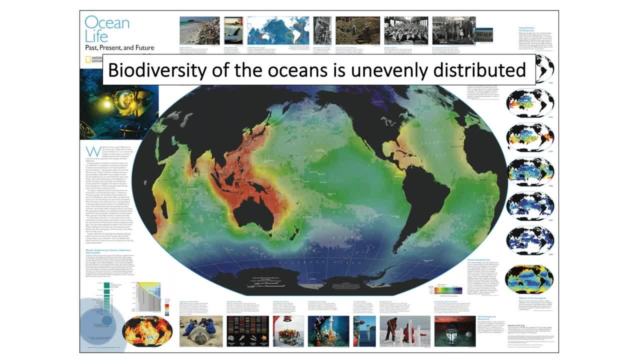 ecoregions by different kinds of taxa and different depths in the oceans. So these are very, very intricate issues and issues that we're making great progress on. Another major issue with biodiversity in the oceans is that the oceans are very, very 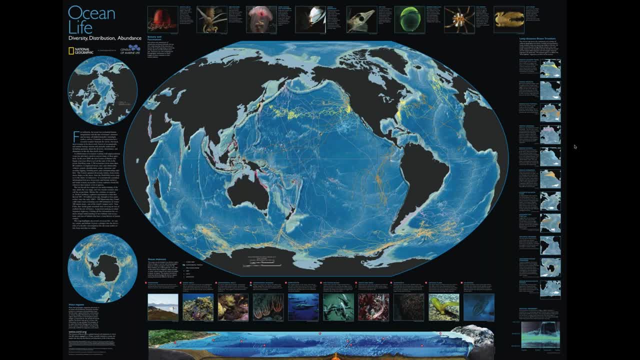 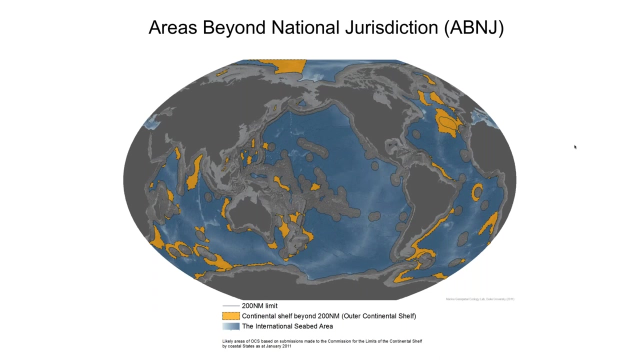 fluid and dynamic, And so we have species that are moving back and forth across the oceans, moving back and forth across jurisdictions, And so many animals in the oceans travel quite long distances across many different ocean basins. Complicating matters even more is the fact that our jurisdictions in the oceans are fairly. 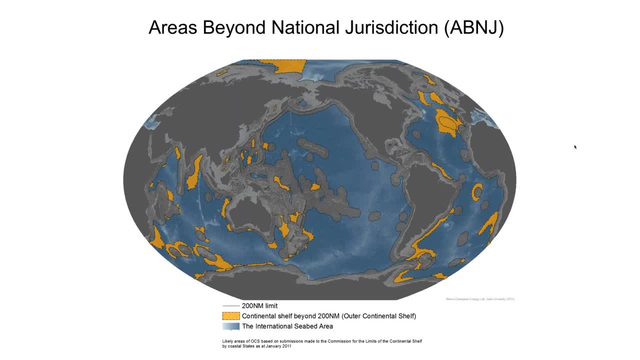 complex. Where we have jurisdictions that are very complex, We have jurisdictions that are very complex. We have jurisdictions that are very complex. We have jurisdictions for national boundaries. We have jurisdictions to the 200 nautical mile limit of the extended economic zones of different countries. 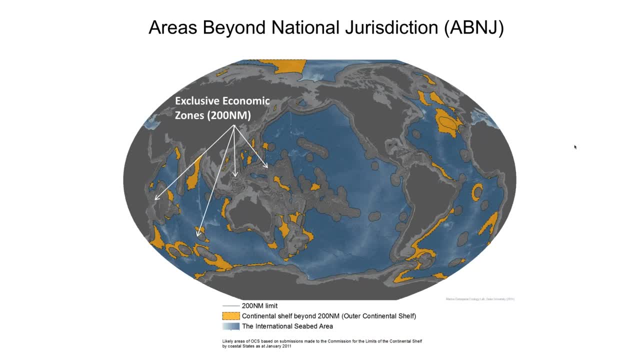 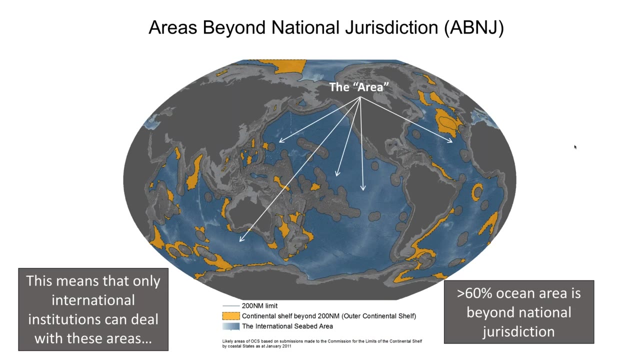 We have continental shelf, extended continental shelf proposals, And so these areas are quite dispersed in our oceans around the world. Sixty percent of our oceans are beyond national jurisdiction, and this is extremely important as we go into discussing a new BB&J treaty, because this means that only international 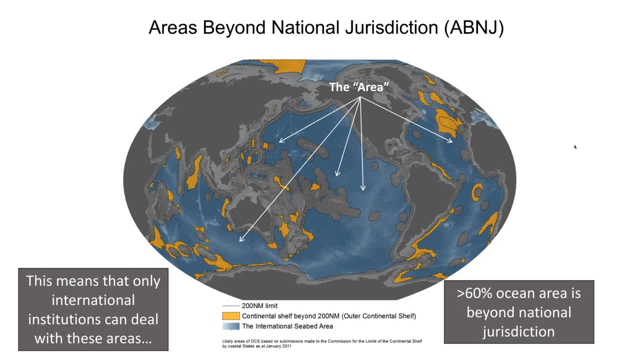 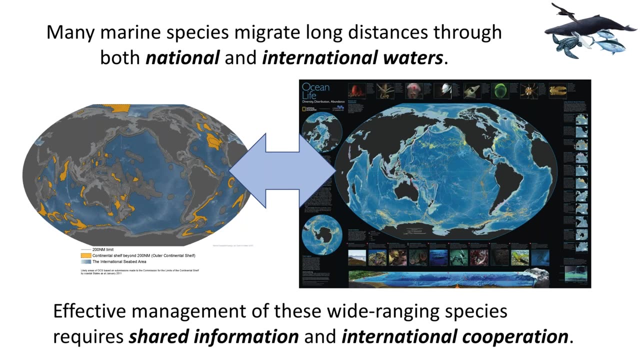 institutions can deal effectively with these areas, And so this is the focus of our topic today- is how do we provide the data and information needed to look at managing these areas beyond national jurisdiction. So many species migrate long distances through both national and international waters, and 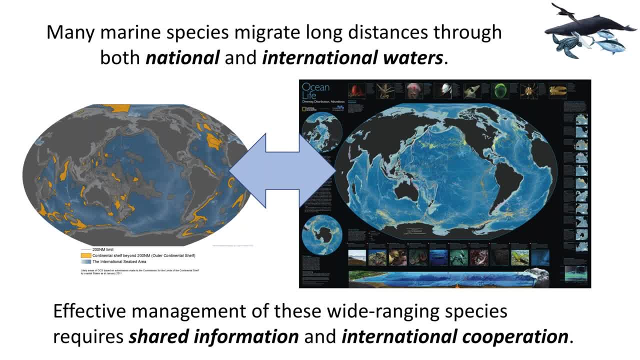 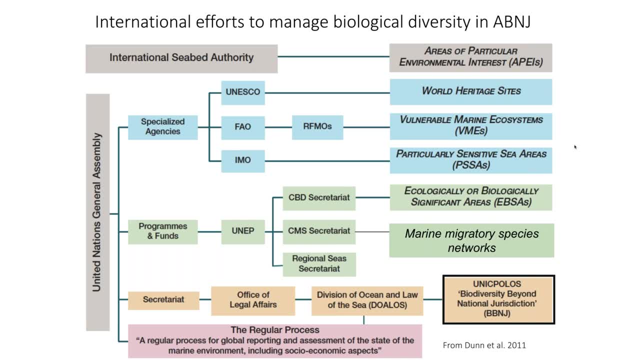 we really need to have shared information and international cooperation. Okay, So let's look at a little bit more of the topics. of the topic: We have a lot of different types of information that we can access for the different waters that we're looking at. 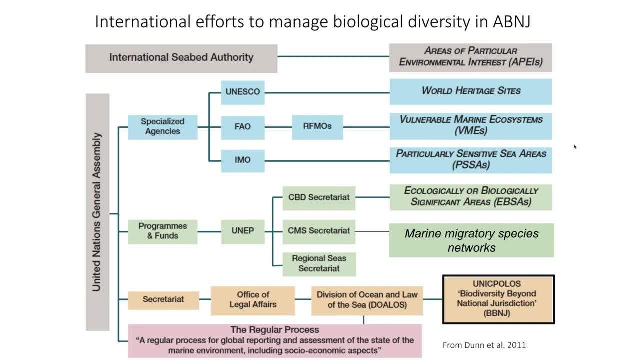 And one of the key aspects of this is theît to be able to effectively manage this biodiversity, various aspects of areas beyond national jurisdiction. The thing that's most important right now, this month, is preparing for the negotiations to be going on in New York coming up in September: the IGC negotiations. So we're 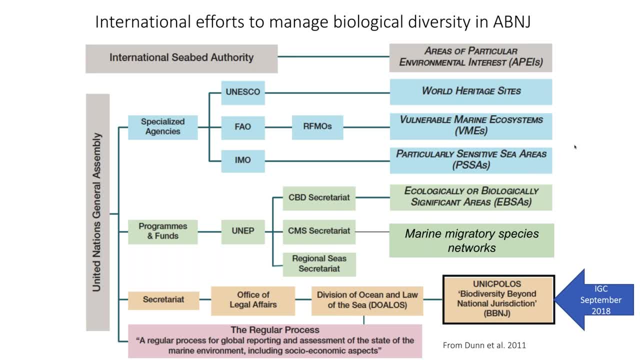 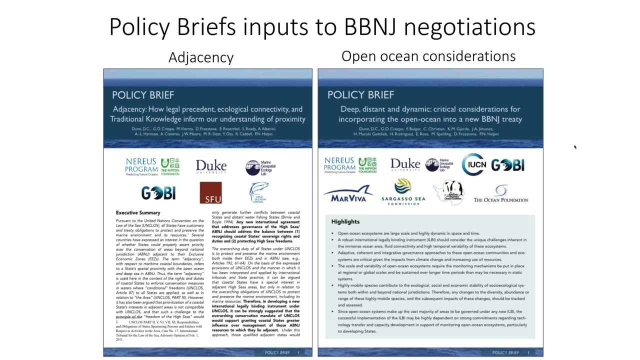 very interested in trying to provide information to the parties going into that negotiation on where do we stand right now in our knowledge base on biodiversity beyond national jurisdiction, Our lab group has worked on several different policy briefs to help support the BB&J negotiations. Two of 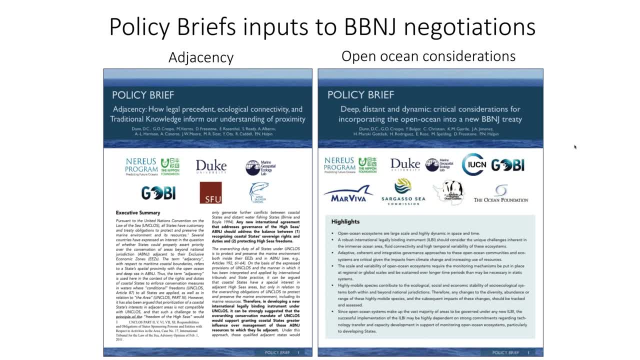 them I have on the screen. here is a policy brief on adjacency issues and another one on open ocean considerations. Currently we're putting together another one specifically on biodiversity data for areas beyond national jurisdiction, and we will hopefully have this developed and ready for New York in several weeks. So we just wanted to advertise this, that we 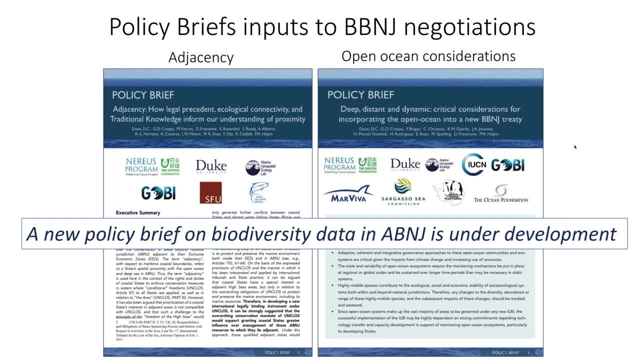 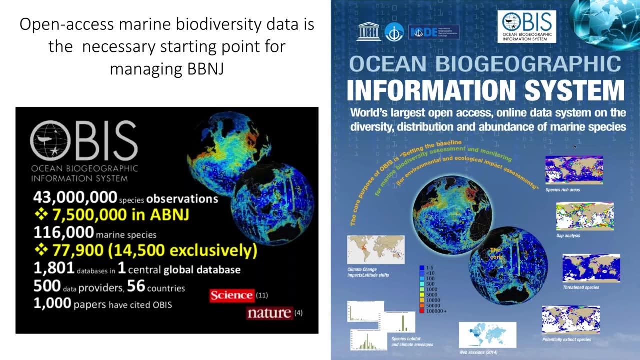 will have this policy brief developed for the New York negotiations, And some of the things I'm going to be speaking about this morning are going to be contained in that policy brief. So the first main point I want to make is that we really need open access marine biodiversity data as the necessary 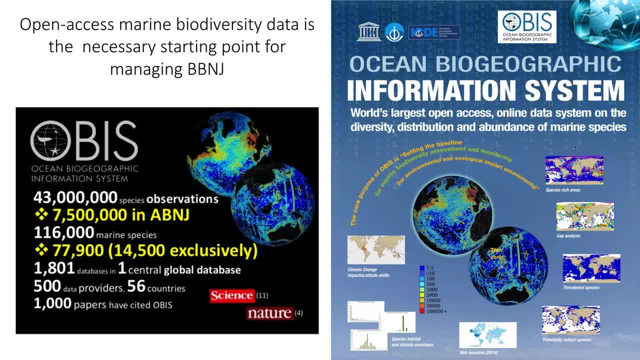 starting point to manage biodiversity beyond national jurisdiction. And this is essential and it's not just having data, it's having data that's openly accessible to all parties and all interested groups and stakeholders to be able to understand and to be able to manage effectively manage biodiversity. 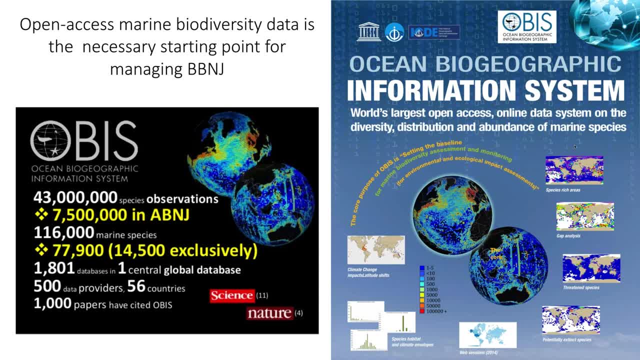 in the oceans. I currently work, and have worked for many years, with the Ocean Bioregraphic Information System, or OBIS, which was started out as an academic exercise under the census of marine life almost 20 years ago. It is now under IOC and is a formal organization in the as an international body. So OBIS is the main. 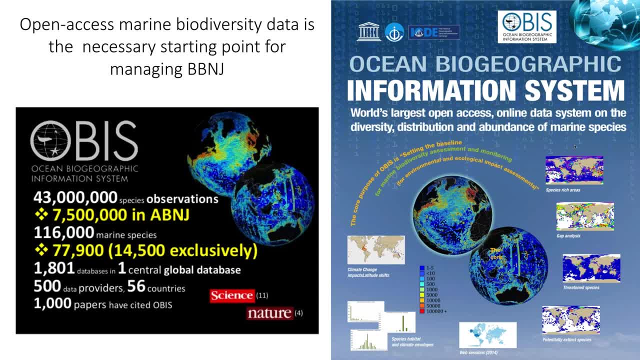 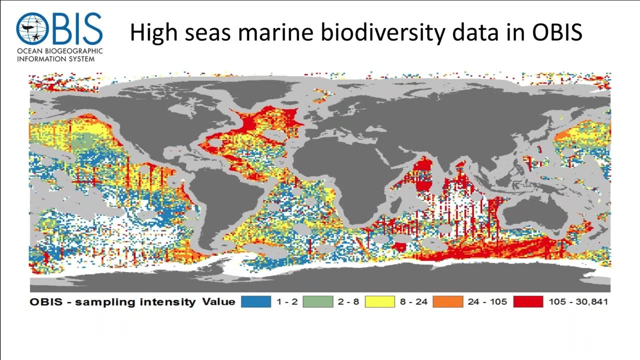 repository for for international data on marine biodiversity and currently has more than 7.5 million records in areas beyond national jurisdiction. This map here is a map of the distribution of marine biodiversity data globally held within OBIS And, as you can see, there's a variety of data there. 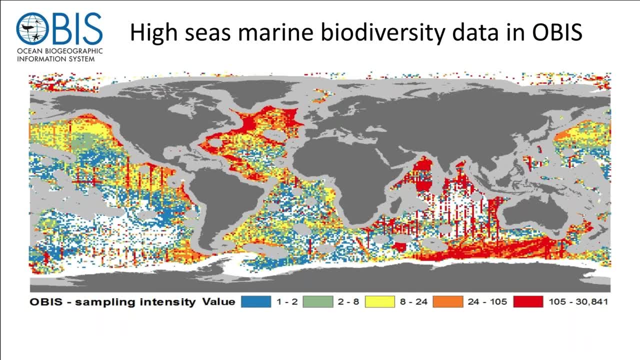 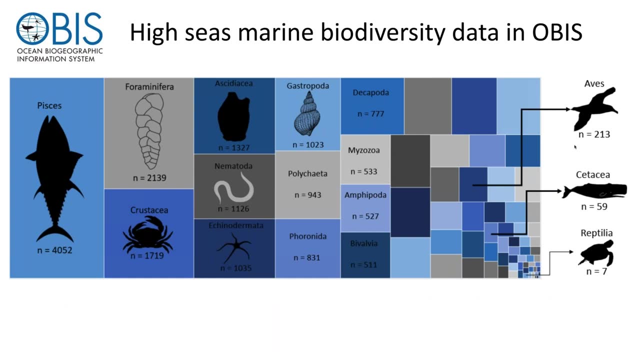 And the hot colors, the red and orange colors, are areas where we have a fairly significant amount of data, and the areas that are blue or white is where we have fairly limited data. So you can see the distributions are not evenly spread around the oceans. In addition to the geographic distribution, we also need to 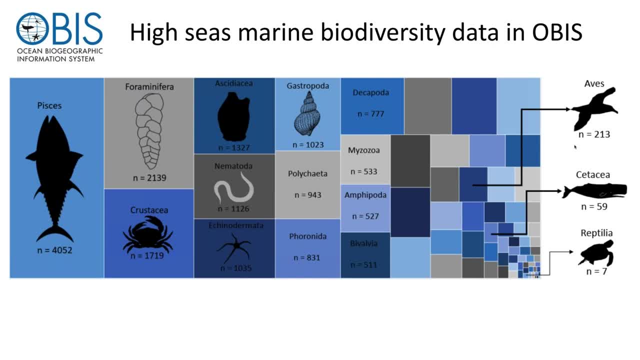 think about the taxonomic distribution of our information and data, And so this graph here is showing the data holdings within OBIS in areas beyond national jurisdiction, And what you can see is that some of the most well-known species, like fish and marine mammals, seabirds, sea turtles, fit. how 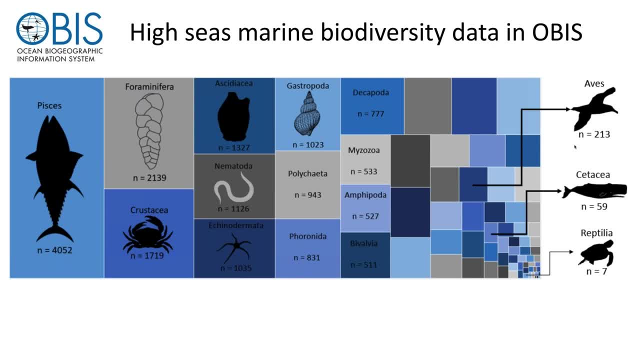 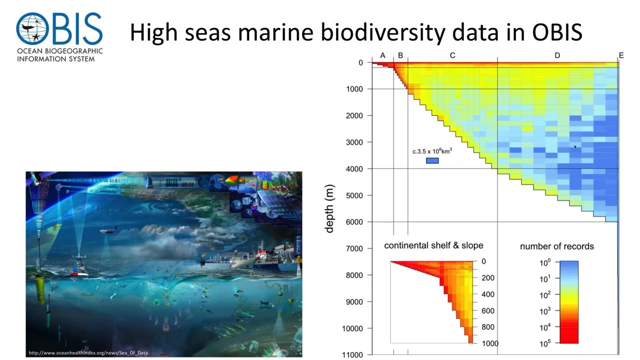 they fit into this distribution, But there's a large amount of biodiversity data that deals with microbes and invertebrates that many people don't consider, And this is the area where we will see the largest growth of new data in the future: The distribution of biodiversity data in the oceans. 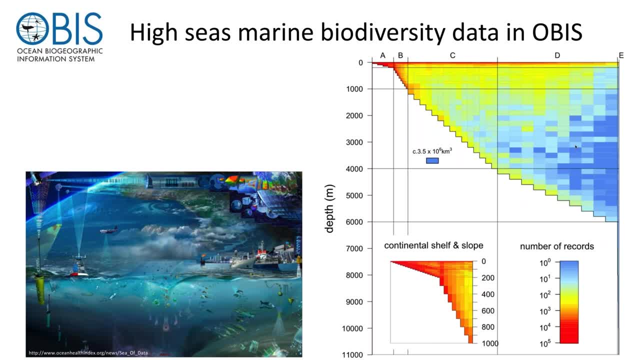 also isn't distributed evenly when we think about the vertical structure of the oceans. So we have our highest density of data holdings near the coast and we also have data holdings at the surface of the oceans. You can see the red thin area there. But what we're? missing data or lacking data, or could. 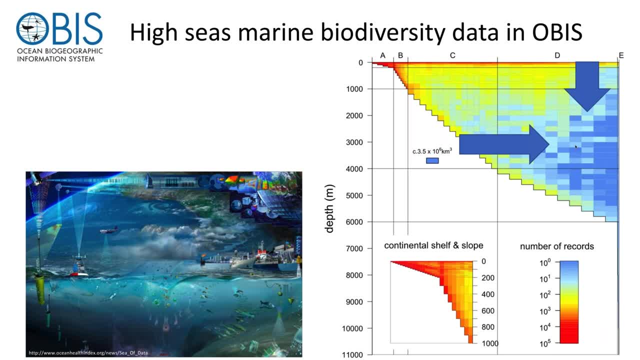 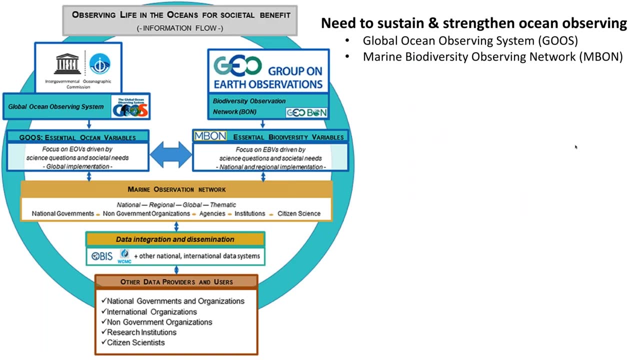 improve on this data is in the far offshore areas and areas in the midwater column and deep seas, So we need to think about the distribution of biodiversity data in the oceans. We need continued data collection in the offshore areas beyond national jurisdiction, in the midwater column and also in the deep seas. One of the points 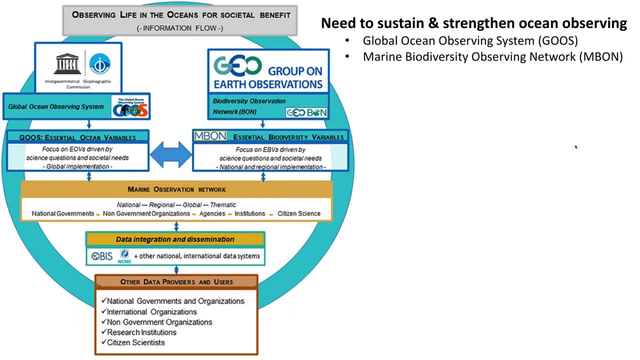 I want to make is that we need to sustain and strengthen the ocean observing networks that already exist, And two of them, the Global Ocean Observing System, or GOOSS, and another, the Marine Biodiversity Observing Network, or IMBON, are two of the observing networks that feed, information and give us guidance on how to do this. So we need to think about the distribution of biodiversity data in the oceans. We need to think about the distribution of biodiversity data in the oceans. We need to think about the distribution of biodiversity data in the oceans. 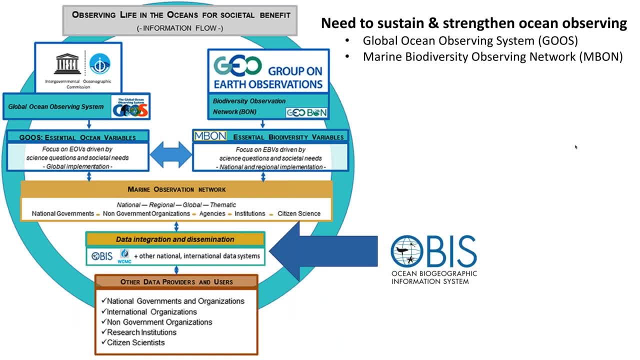 guidance on how to collect and normalize information to be used in areas beyond natural jurisdiction. OBIS is the main repository of a lot of this information, once it's collected. So the point I want to make here is that we need to properly strengthen and support an existing international infrastructure, and I 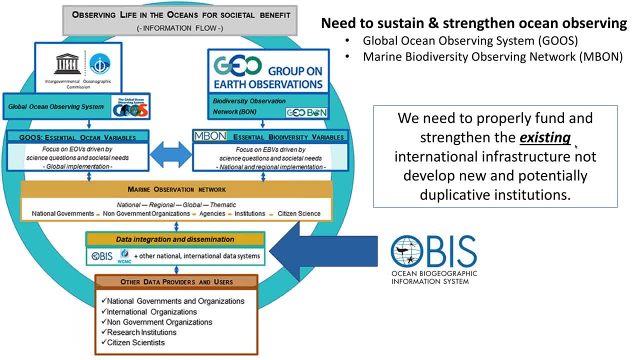 really think we should do this instead of developing new or duplicative institutions. We already have the infrastructure, but it needs to be reduced. We need to continue to support infrastructure and keep the places that are kind and safe needs to be strengthened and supported into the future, and this is something I 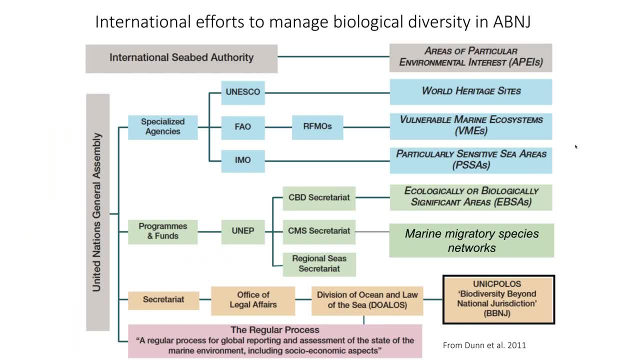 think should come out in the BB&J negotiations. In addition to the BB&J negotiations, there have been ongoing work with biodiversity in areas beyond national jurisdiction. One significant area has been the efforts under the Convention on Biological Diversity, designating and defining ecologically or 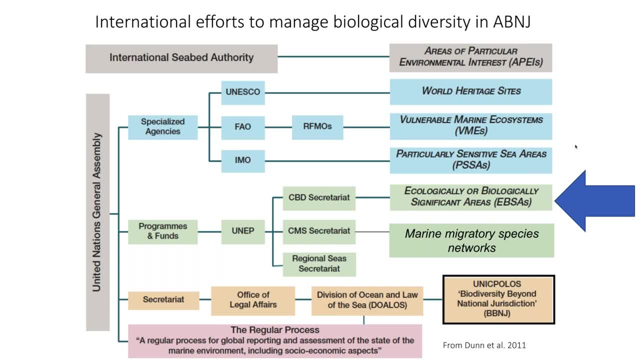 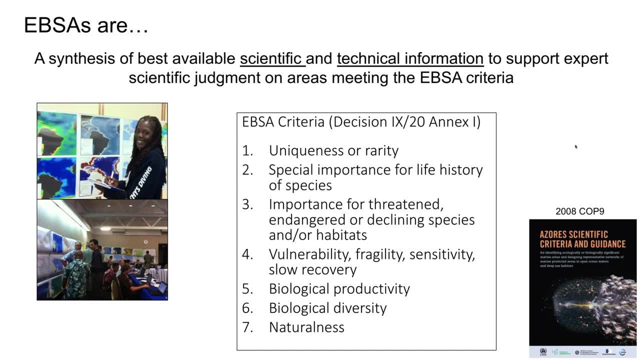 biologically significant areas, or EBSAs. Our group has been involved in this process since the origin. EBSAs are a synthesis of available scientific and technical information to support scientific judgment and the application of the EBSA criteria. These have been conducted through regional workshops. 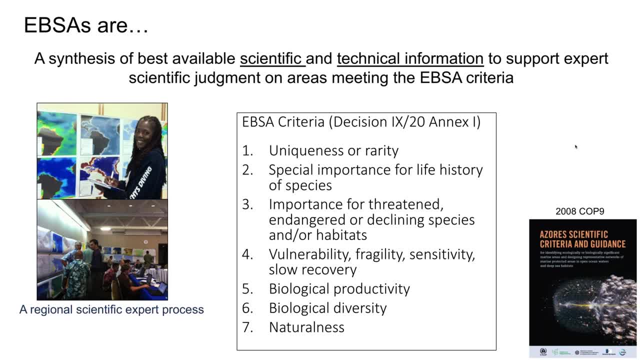 over the last decade. These are regional scientific expert processes and there are seven criteria that can be described for areas beyond the Convention on Biological Diversity. EBSAs are a synthesis of available scientific and technical areas that meet these criteria and are defined or described as: 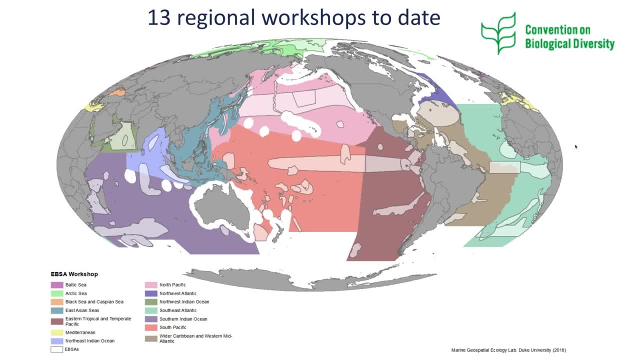 ecologically important. There have been 13 regional workshops to date and we are currently looking at ways to review and revise existing workshop regions. I just returned two weeks ago from meetings in the African region, from Angola for the Benguela Current, where we were looking at potential revisions and updates, and 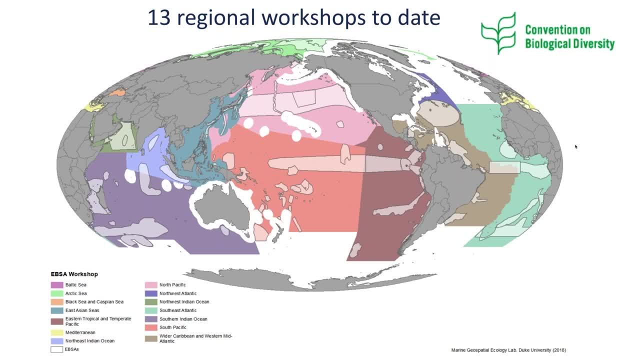 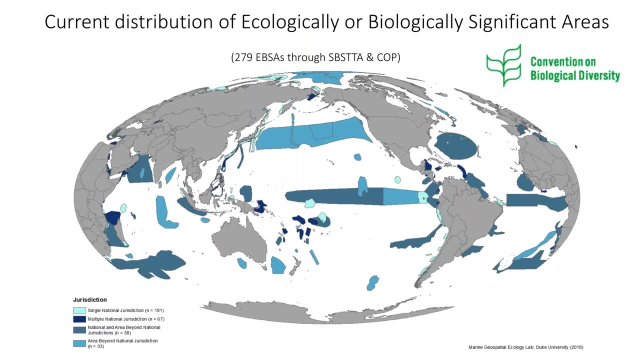 improvements to the EBSA criteria. This is a very interesting time now to be refining and further developing the EBSA process. To date, there are currently 279 EBSAs that have been described. globally, There are 319 that are in process. So, in addition to the 279, the total number is 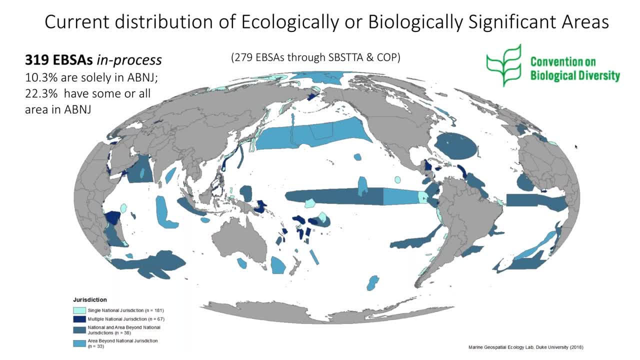 319.. These have gone through SUBSTA and some remaining EBSAs need to go through the COP meeting coming up in Egypt. Of these, over 10% are entirely in areas beyond national jurisdiction and 22% have some or all areas in national. 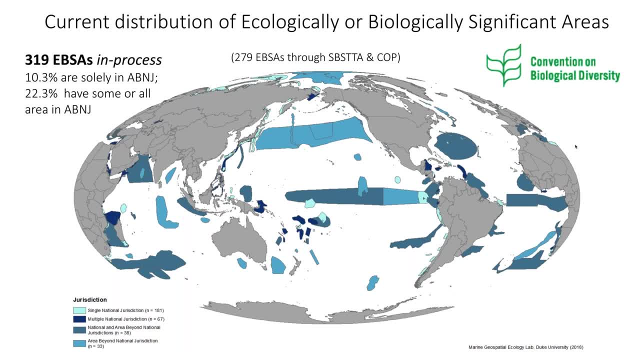 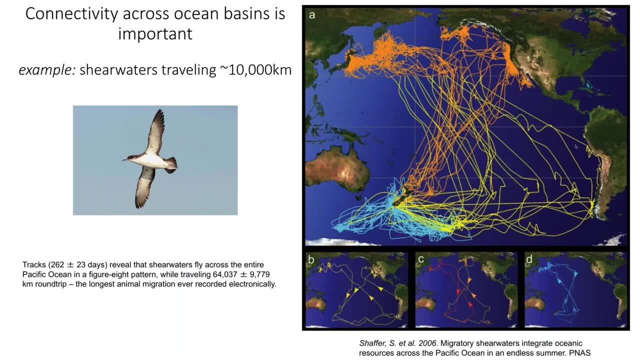 jurisdiction beyond national jurisdiction. Some of the largest EBSA sites are in the areas beyond national jurisdiction- the large oceanographic areas. Another point that's very important in going into the negotiations is that connectivity across ocean-based migration basins is extremely important. This is showing just a diagram of sheer water bird. 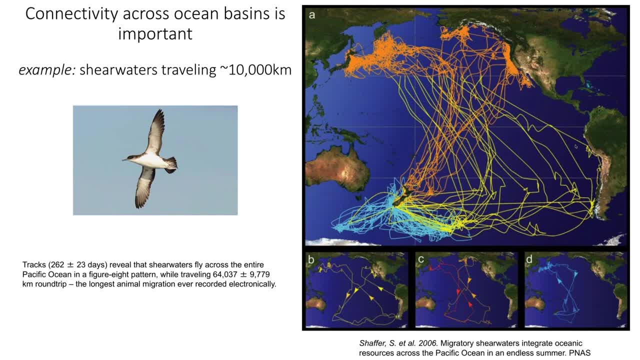 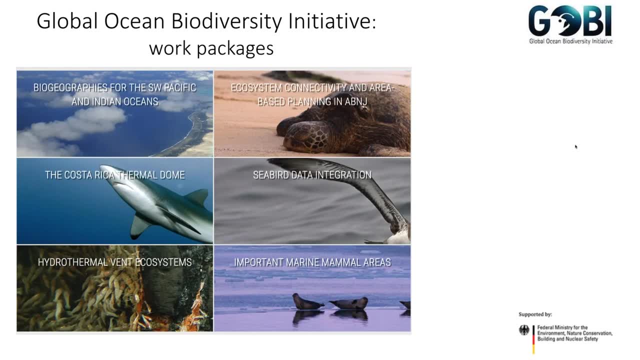 migrations in the Pacific, showing individual animals traveling across the entire Pacific Basin from the southern hemisphere to the northern hemisphere and back. There are three work packages ongoing right now with a project under the Global Ocean Biodiversity Initiative that are looking at issues of migratory animals. These projects 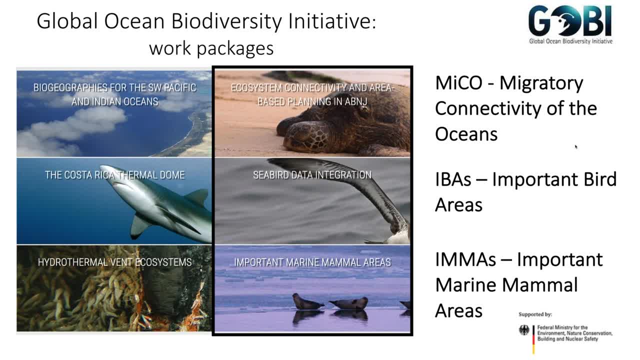 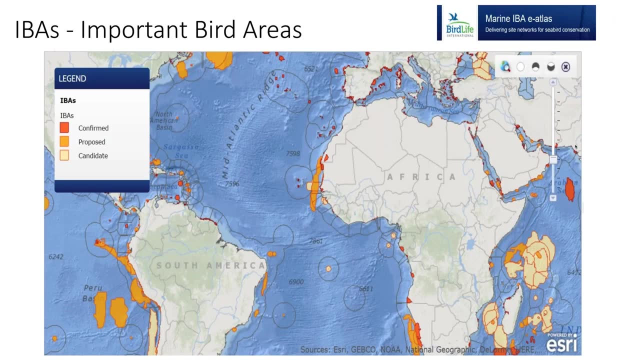 include the MICO project, Migratory Connectivity of the Oceans program, the IBA's project on important bird areas and the EMMA's project looking at important marine mammal areas. I just want to very briefly highlight these projects. So first, the important bird areas. 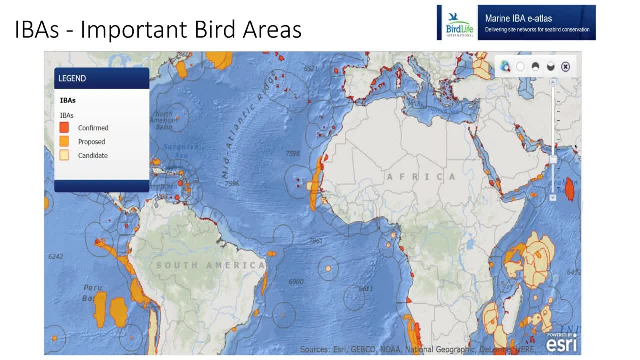 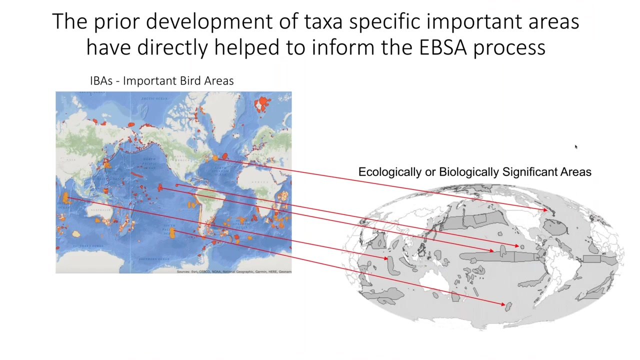 project is looking at synthesizing information on seabirds around the world to help inform international processes- and this is extremely important- on trying to synthesize this information for use in management and also the description of ecologically or biologically significant areas. So these IBA's important bird areas have been used effectively in informing the 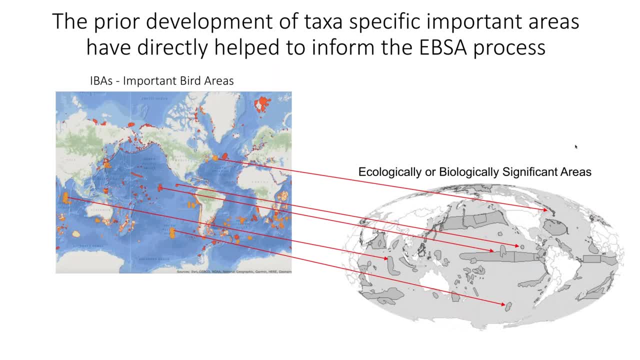 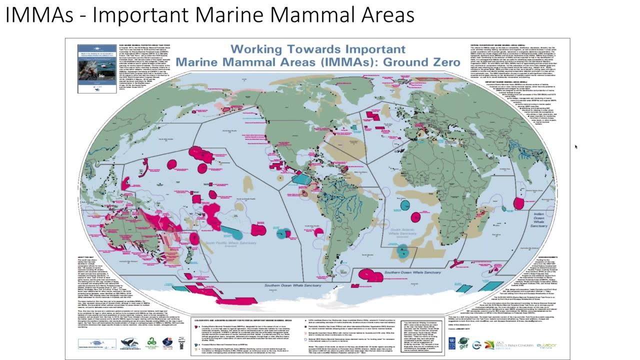 CBD, ecologically or biologically significant EPSA process, by providing information that can be brought into those global workshops that's already been synthesized to show these are important areas for seabirds. Similarly, we're looking at, you know, the development of important marine mammal areas as a way to also get the scientific community. 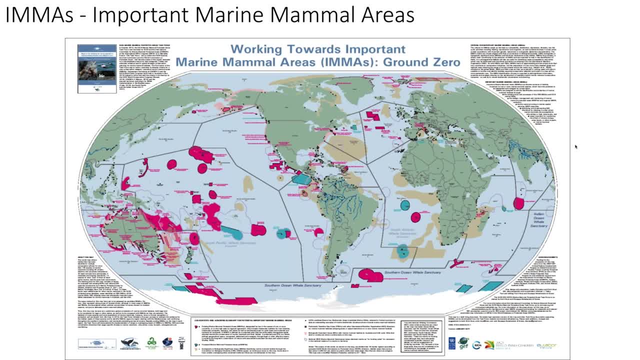 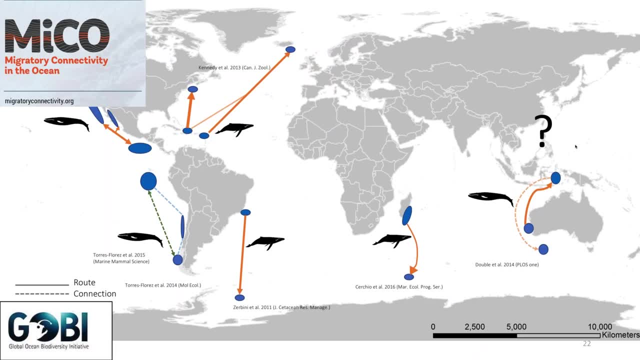 the specialists in marine mammals to describe areas that are of special importance for those species. Finally, the third project in this cluster of projects called MICO is one that's being conducted in our lab, and this project brings together many, many researchers from around the world to look at the connectivity of important ocean areas, And so this is not just looking. 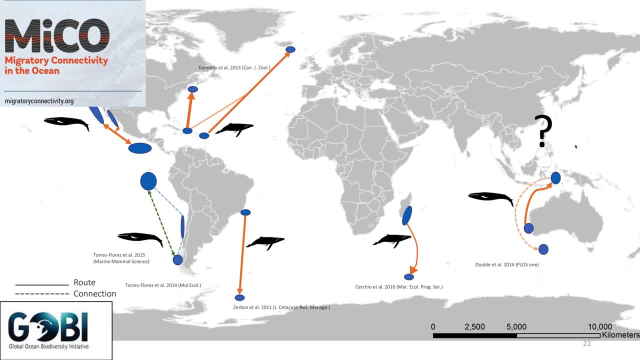 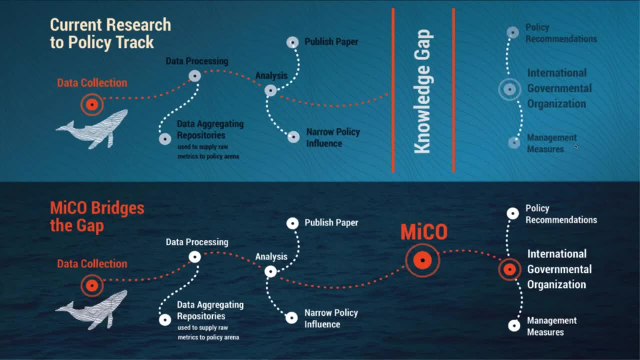 at the places where we find the important animals, but also the connecting routes that connect them, the pathways and corridors that connect these species. So this MICO project tries to fill the knowledge gap of looking at where we're finding information on the oceans of important areas and the connections between them, and trying to bring that information. 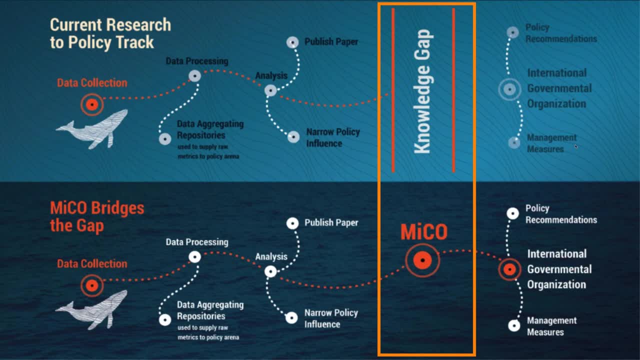 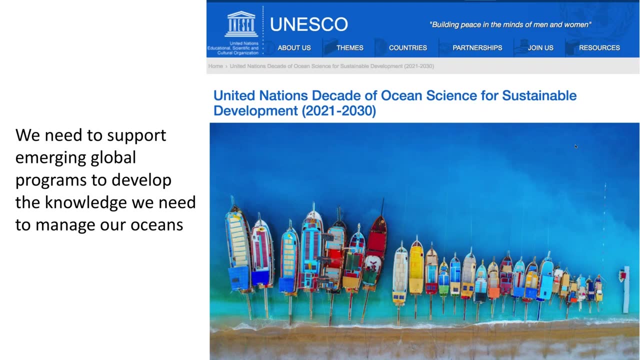 directly into the policy and management arena. Finally, we're looking at the resources that we're taking from the pathological agencies. one of the things looking into the future is the need to support emerging global programs to develop the knowledge to manage our oceans, and so one, not the 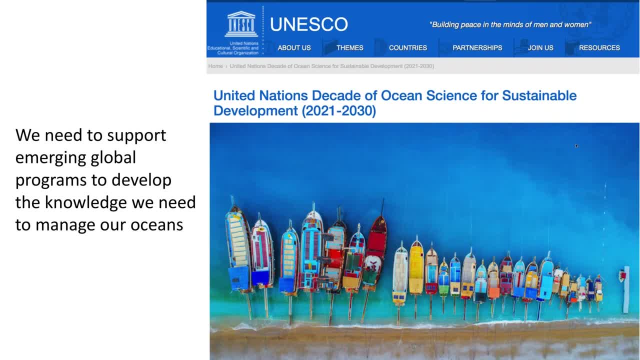 only one, but one that we really want to highlight is the emerging United Nations decade of ocean science. this is something that we feel could be very important to try to broaden our knowledge base and our information and synthesis of information to directly provide new data to help support. 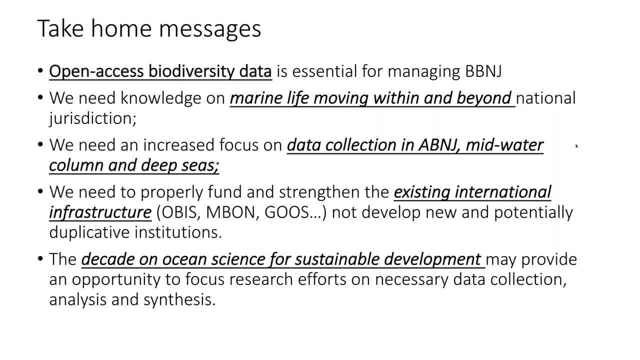 biodiversity management beyond national jurisdiction. so to recap take-home messages: we need open access biodiversity data, which will be essential for managing biodiversity beyond national jurisdiction. we need knowledge on marine life moving within and beyond national jurisdiction. we need an increased focus on data collection in areas beyond national jurisdiction. in 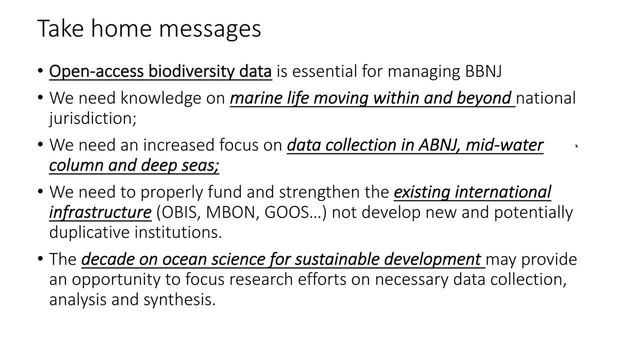 mid-water columns and in the deep seas. we need to properly fund and strengthen the existing international infrastructure and institutions- not develop new institutions but to strengthen the ones that already exist- and we need to look at the decade of ocean science for sustainable development as an opportunity to focus research efforts on necessary data collection, analysis and 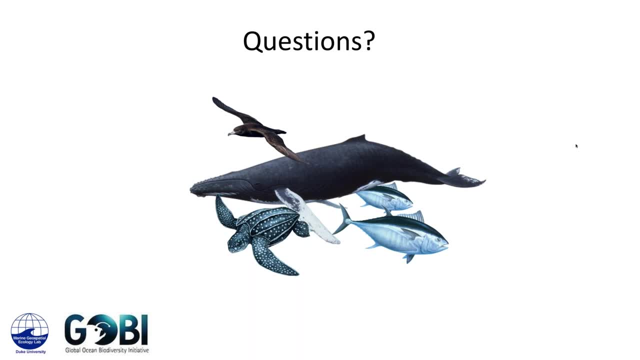 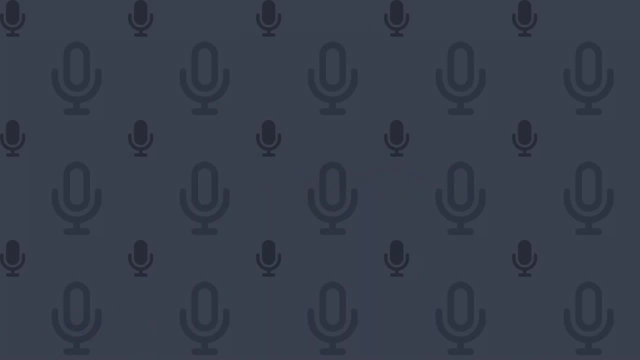 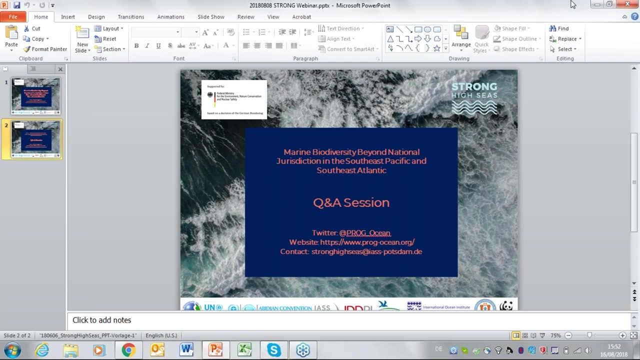 synthesis, thank you. thank you, professor. we have one question. I hope you can hear me. we have a few questions. the first one is in regard to OBIS. the question is: does it have the IT and human resource capabilities to handle additional data that you predict would be generated and also does always have the capability to connect with other? 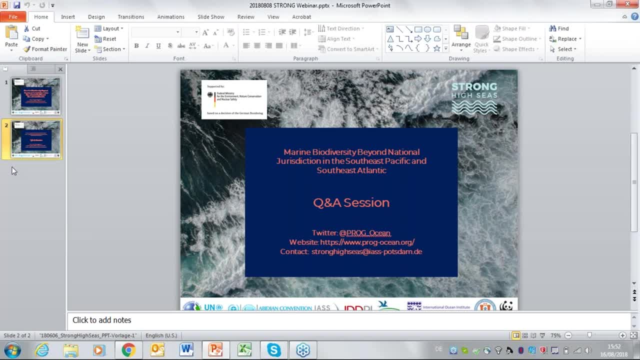 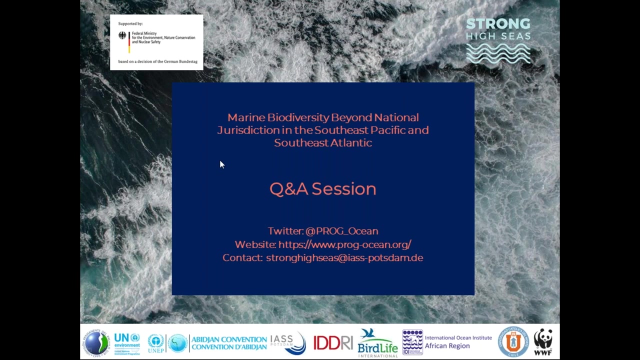 existing databases and does it have capabilities to harvest it? okay, it's an excellent question. though, is a consortium where there's a central repository that's under the iode offices of ioc, unesco, ioc in belgium, in austin, belgium? um, there are a number of geographic and thematic nodes, our lab. 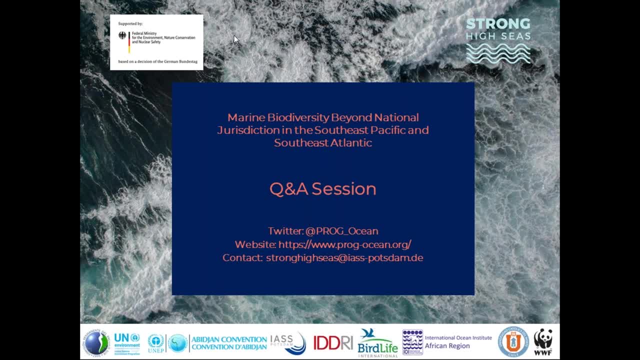 runs what's called opus cmap, which is the node, international node- for marine mammals, sea turtles and seabirds, the migratory species. so we've organized that data and then we give that data to the main international program in belgium. we, these areas are need more funding. they. 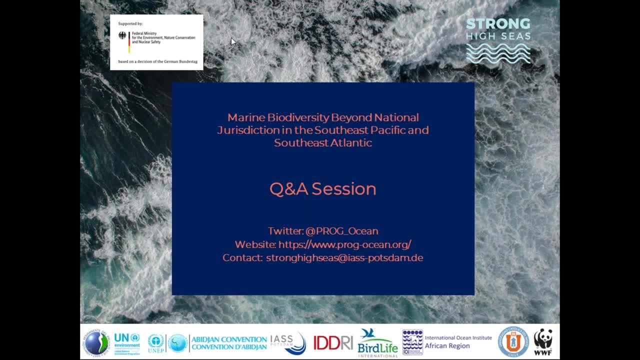 need more resources, but the infrastructure is there. the human infrastructure of different organized groups in different regions around the world and scientists does exist, but as we move forward, we need to get increased resources and more stable funding to keep this moving forward. so my main point is that the infrastructure is. 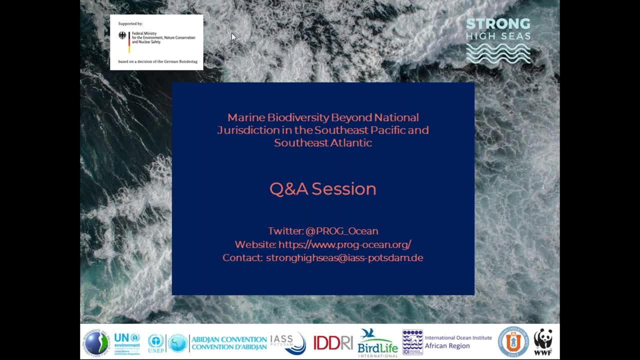 there. we just need to support it in a in a better way. okay, excellent, thank you. so we have a few more questions coming in. this one is in regard to believe you said something in regard to not creating a new institution. I'm not sure if you could maybe explain or clarify what this was in regard to or what you meant by. 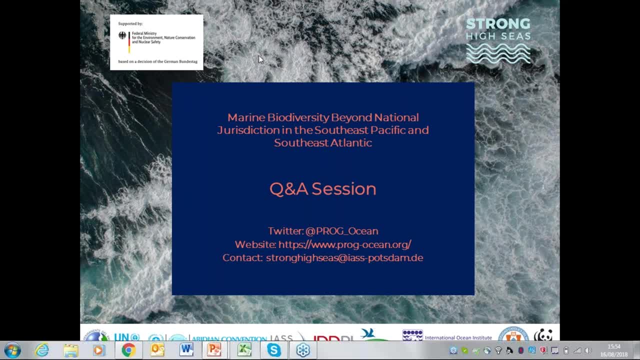 this one. yes, I mean, this was a personal opinion here on. I think there's been quite a bit of repeated movement in the past, when people get excited about a new opportunity to develop new data and they want to create a new system, a new network, a new website. 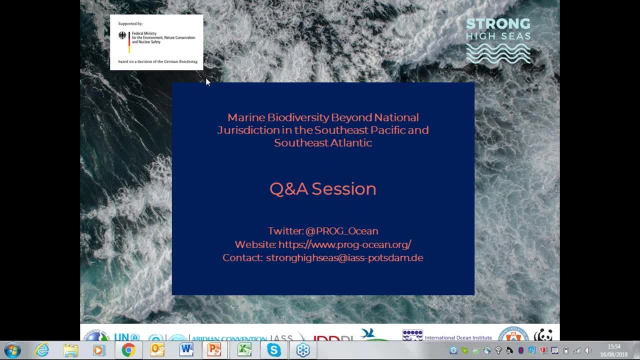 and my point is that many of the existing, the existing infrastructure is already in place. we just need to organize it and fund it and increase the capability to and the usage. and so all too many times I see funders supporting the development of a new site without going on to supporting the existing locations. so I 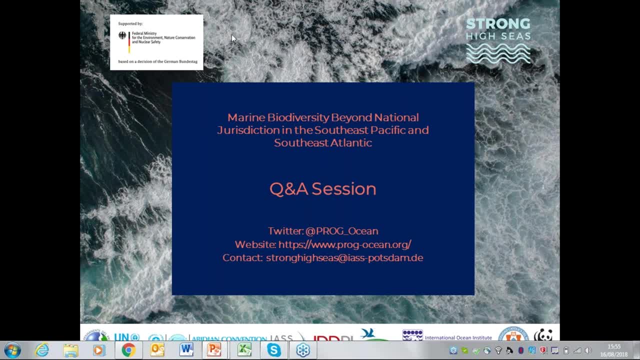 think we're at a point right now where it could be very powerful to to take the existing infrastructure globally on ocean observing networks, OBIS, other tools- and to be able to look at developing these warehouses of data and to to sustain them and to increase access instead of inventing another. 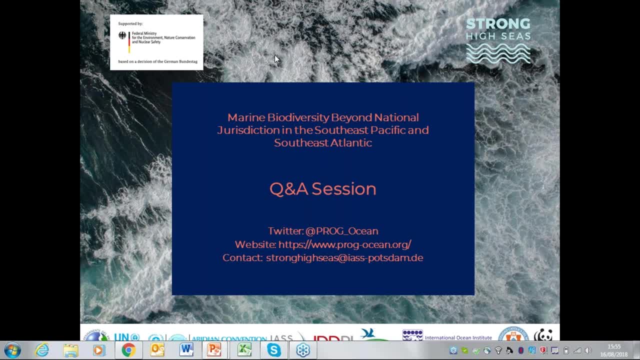 process on top of that. so that's that's my main point. okay, one last question and we go to the next presentations, so this one is for you: how, how to link the various sources of data together so that users know how to find them. there is a. 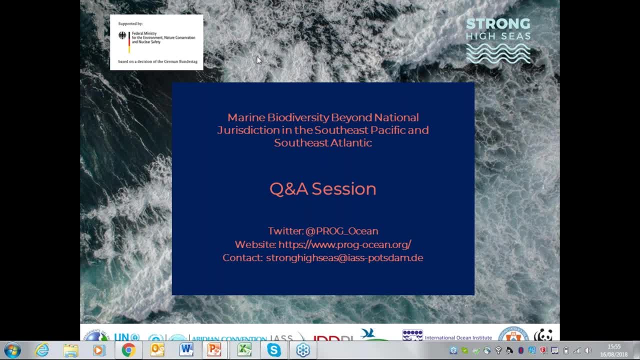 there are ways to link the different data coming through different sources, so there are a variety of different data types. so OBIS brings together the biological observation data. there's already world data centers that exist for oceanographic data, so there's many existing data centers and many of these. 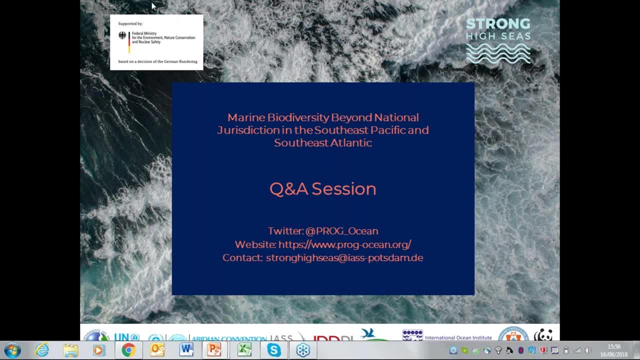 could be linked together. they. you know the. it depends on the project activities. most of the more modern programs that we're working with these days tend to use are starting to use web services and other kinds of techniques to be able to link information through internet services instead of having people you. 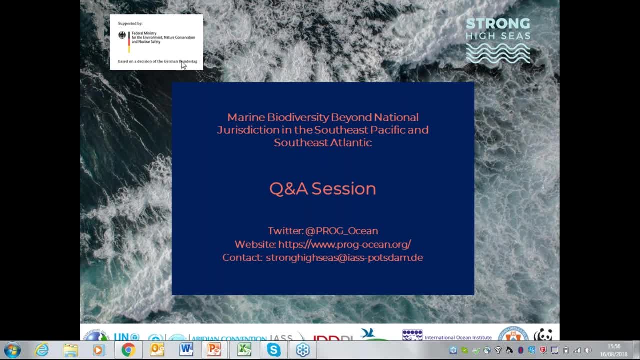 know, have to download individual data files when they want to use them. so as we move into a more interconnected age, it's actually providing these internet services that are extremely important. so so there is a lot of technical activity that can be done to help strengthen the usage and synthesis of this type of information. okay, excellent. 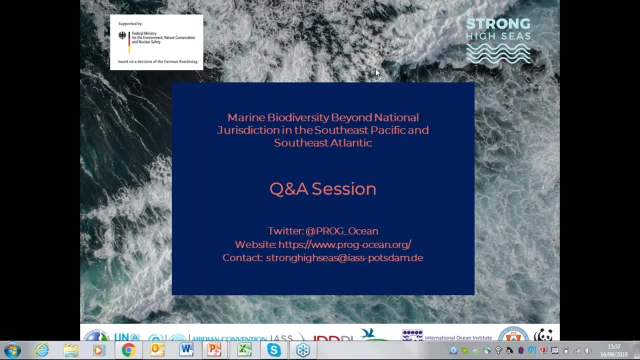 Thank You, professor help. so that is gonna end our Q&A session for the first presentations and we had a few more questions come in here in the during the Q&A, so we'll get back to those during the Q&A session after the next two, two presentations, if we have time, which we 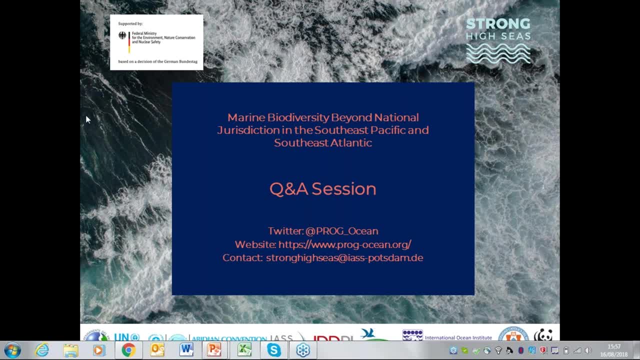 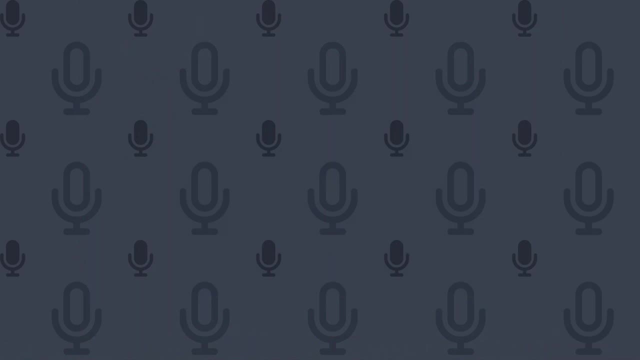 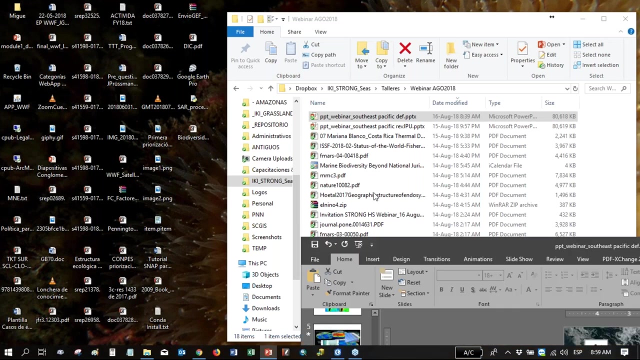 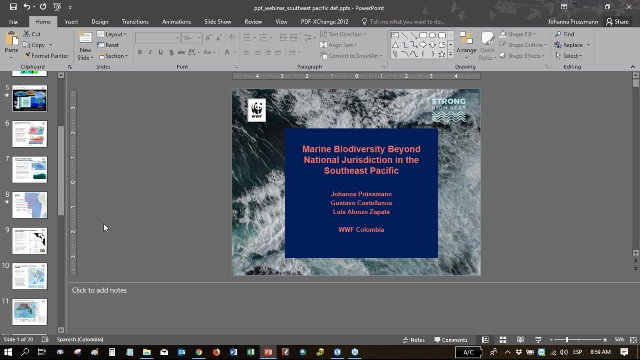 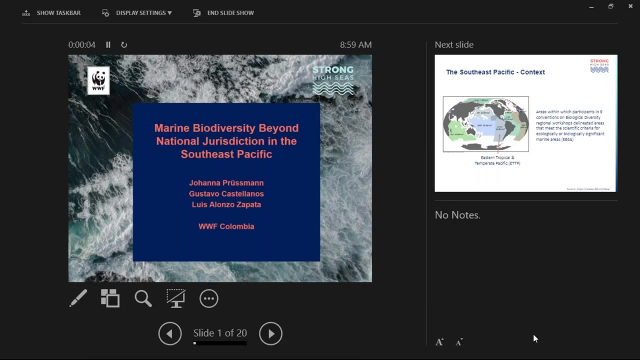 should. so we're now going to hand over, hand it over to Johanna Prussman from WWF Colombia, to make a presentation on marine biodiversity, focusing specifically on the southeast Pacific. give us a few seconds to see. OK, hello to everybody. a? are you able to see my screen properly? yes, we. 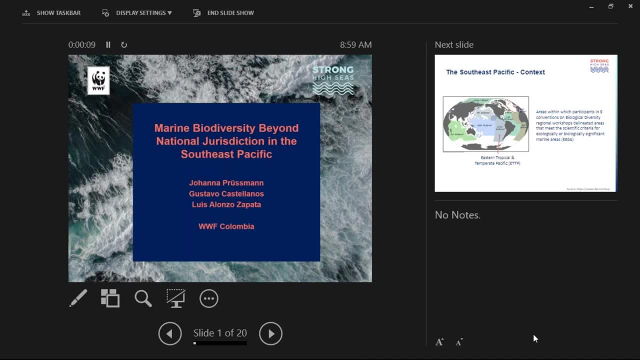 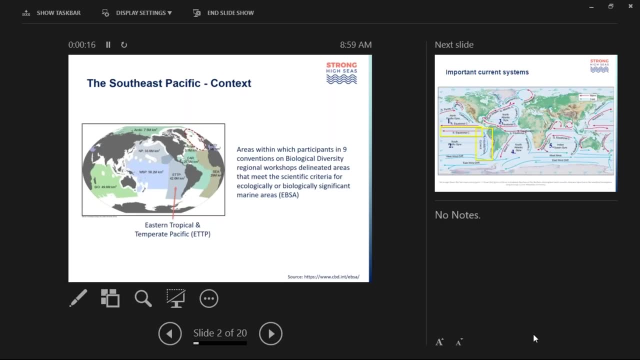 can see it ok. so I'm going to speak a little bit about marine biodiversity beyond the national jurisdiction in the Southeast Pacific region, which is located along the coast and along the Western Coast of the Pacific region, which is located along the coast and along the Western Coast of the. 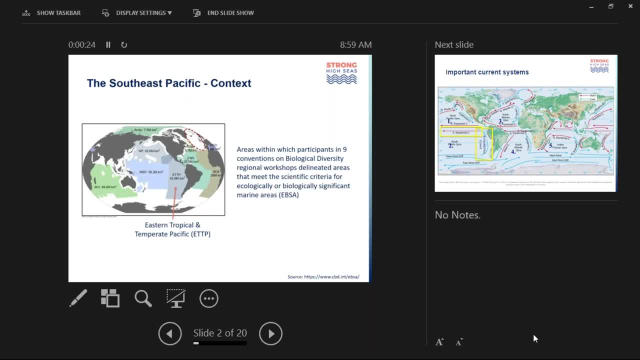 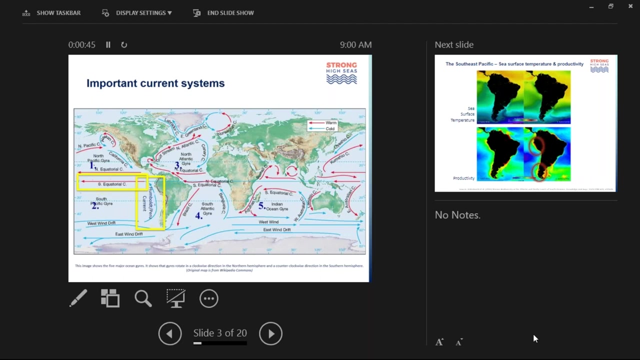 of South America and Central America, ranging from Mexico until Chile. It covers around 42 million square kilometers. Okay, sorry, So it is composed by, is covered mostly by the South Pacific gyre, And the most important currents that cover the area are the Humboldt. 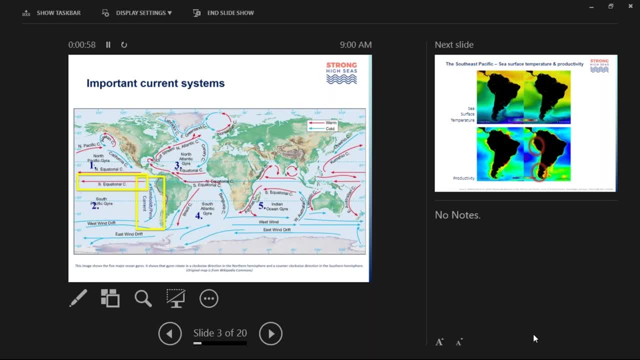 or Peru current that goes from south to north along the eastern part of the Pacific Ocean And it is very important ecologically and biologically because it brings cold waters filled with a lot of nutrients from the cold Antarctic waters to the equator, And also the south equatorial current that goes from east to west along the equator. It is also 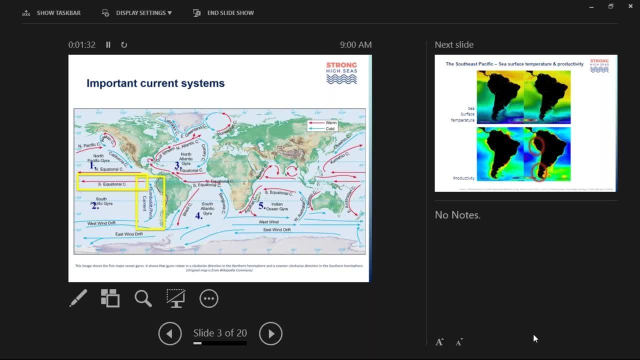 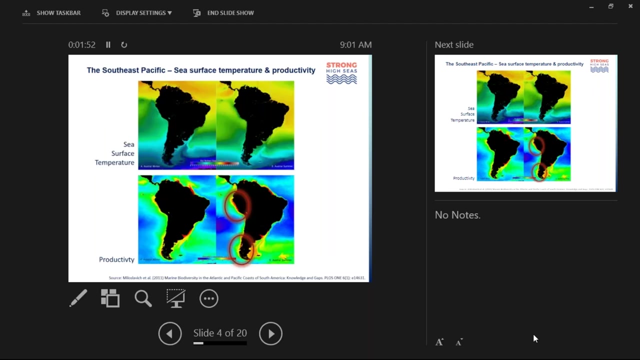 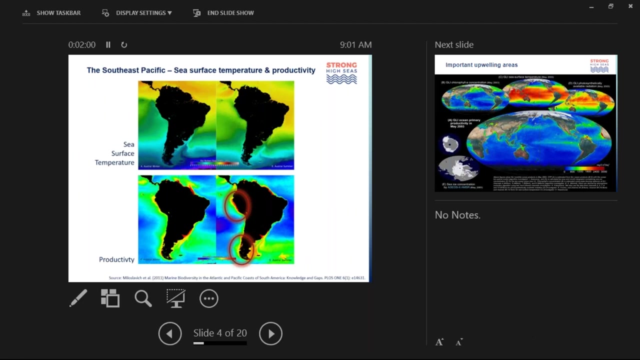 a very significant current because it also transfers a lot of energy along this region and it has also climatic implications regarding the El Nino phenomenon and other atmospheric phenomena. Okay, thank you. Okay, so if we see at the sea surface temperature, it is there is a lot of correlation with the 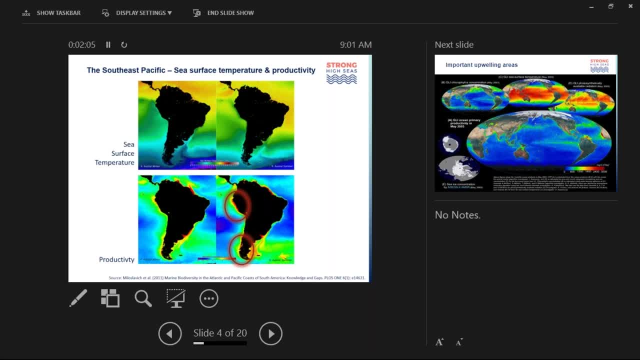 productivity along the coast of western South America And, as you can see, in the austral winter the cold waters from the Arctic Pacific go from the east, from the south to the north, bringing a lot of productivity along this coast, but mostly during the the austral summer. 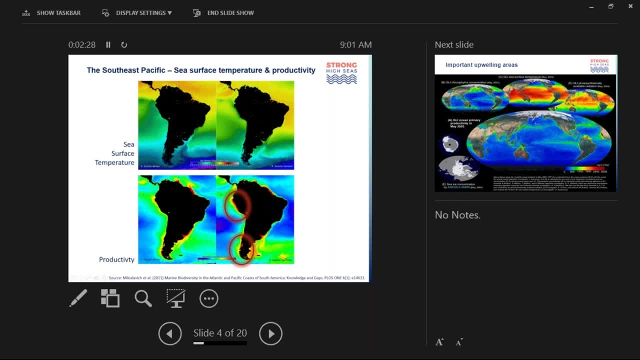 this is very the productivity is really really high, And this is not only because the Humboldt current, which is of course very important, but there's also another phenomenon that causes for disc productivity in mostly in Peru and Chile to be to be veryrative. 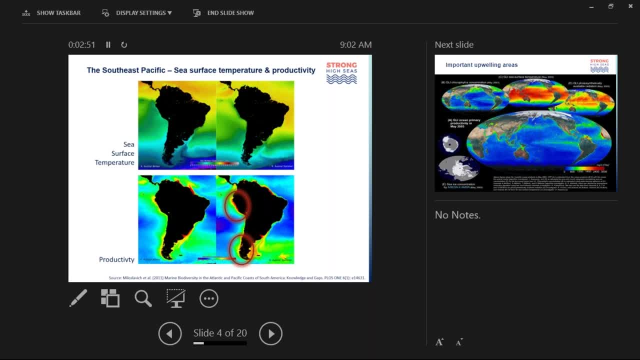 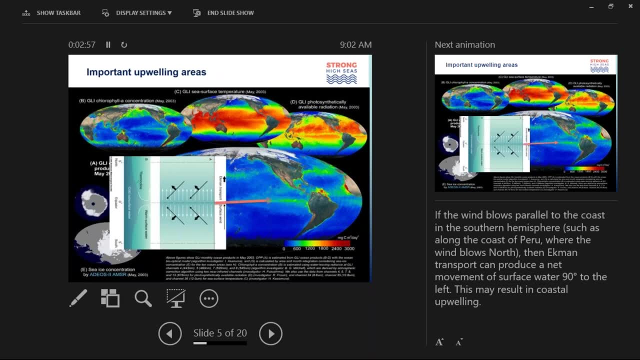 very important and it's called surgence, and it's a mechanism where the cold waters, well the, the circulation of the of the earth moves the water in in in a way that um warm water on the surface is replaced by cold water from the from the bottom of the ocean, bringing also a lot of nutrients. 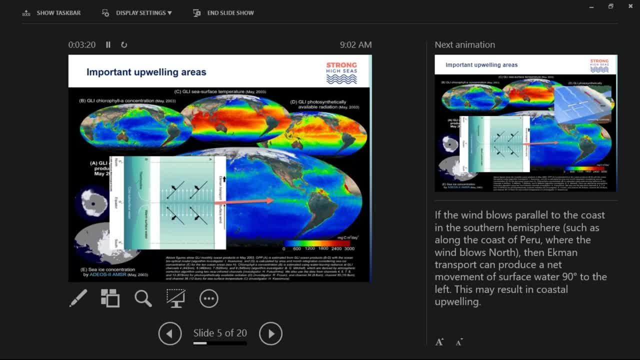 and important- okay, yes, in important uh- characteristics for the um food chain in these are, in these regions there is there are two main um phenomenon of, or ways that the this disurgence is happens. one is along the equatorial current, which which i just showed you, and um it's along. 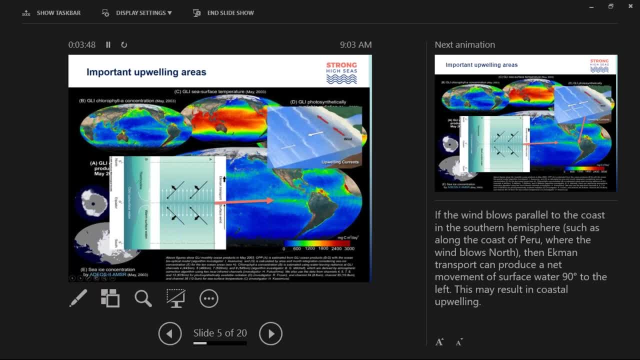 along this, this region, where whereby, by the rotation of of earth, the waters kind of separate and the words on the surface. so one cold water from the, from the bottom of the ocean, comes and replaces this one water that is flowing in the northern hemisphere to the north and in the southern 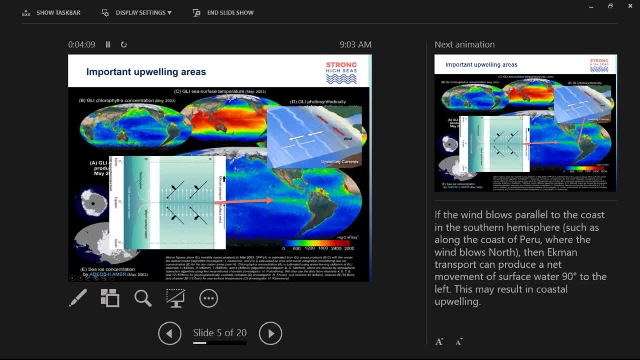 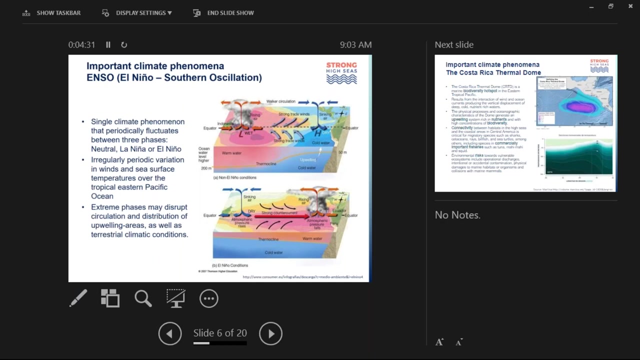 hemisphere, to the south and also along the coast of peru, ecuador and the middle of colombia, there's also a cooled heath, Amur surวยla, a world previously a very important phenomenon across this region and that will outside each surface also contains a current which is 32 days of cock. Belgia啊, another very important. 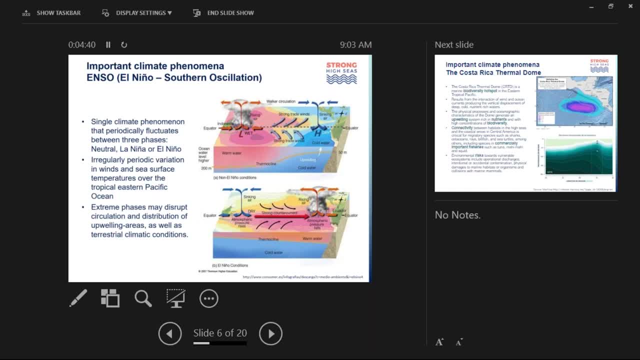 phenomenon along this region is the denso el nino and so southern ocean oscillation, and this is this phenomenon that periodically fluctuates in between three phases: it has normal conditions, weakening conditions, which is El Niño, and it has stronger conditions, which is La Niña. 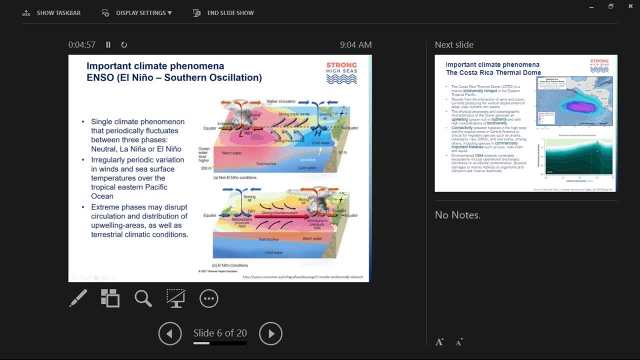 It is driven mostly by the trade winds that flow from the west to the east, But when these winds are weakened, that's when we have these warm waters that are usually kept in the western part of the Pacific Ocean by these trade winds, since they are weakened. 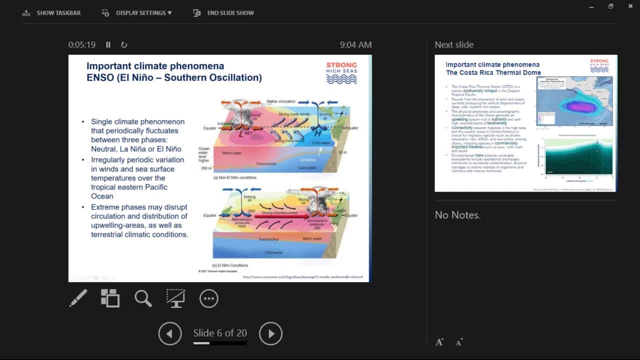 they come over to the equator, bringing wet conditions to a region that is mostly it's very renowned for being very, very dry. Along these coasts is the Atacama Desert, one of the driest regions in the world. But when the trade winds are weakened, all this warm water from Australia brings very 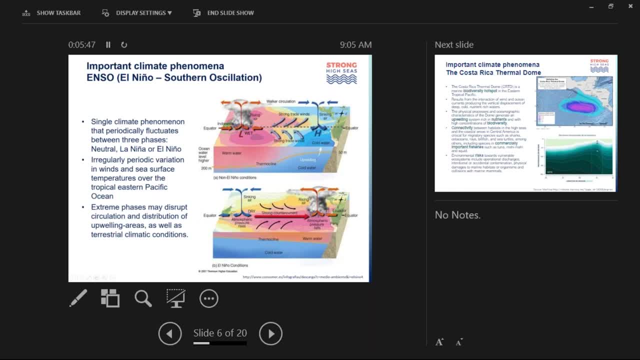 wet conditions along these coasts. However, on the other side of the Andes, mostly in Colombia, then we have very, very dry and hot periods. So it is very interesting how these processes affect not only the climatic conditions of the region but also the runoff from rivers, and that changes the biogeochemical cycles. 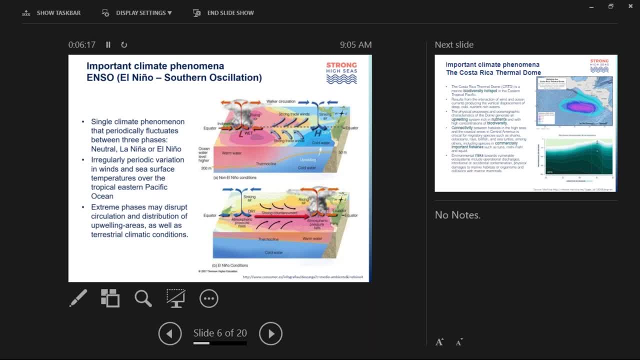 along this coast. So mostly the food change is weakened to the El Niño conditions because the fauna also has to go deeper, because, as you can see here, the thermoclean deepens, So the fauna has to go a lot deeper And also the runoff makes for the salinity of the water in this region to be lower. But during La Niña Condition they have a great deal of water in this region And also the runoff makes for the salinity of the water in this region to be lower, But during La Niña Condition they have a lot of water in this region. 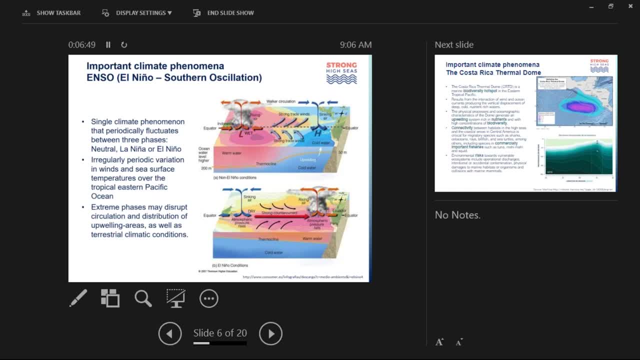 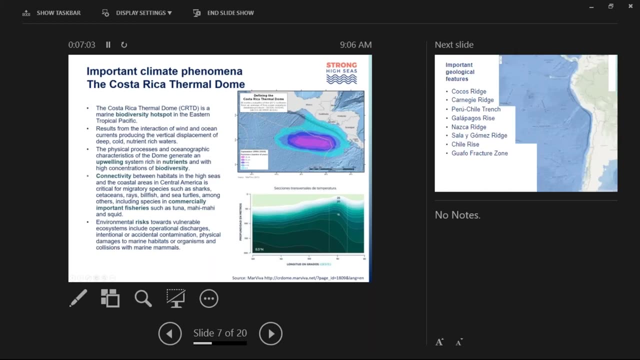 usually the effect is contrary, and then the thermocline will be more shallow and then we will have a lot of primary productivity along the coast. Another important climate phenomena is the Costa Rica Thermal Dome is another resurgence area along the western coast of Mexico, Guatemala, El Salvador, Honduras, Nicaragua and Costa Rica and it brings a 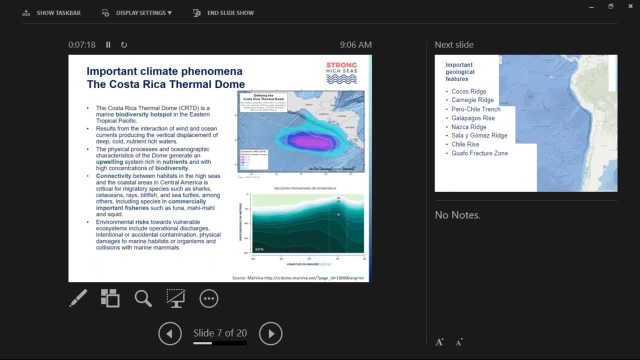 lot of nutrients and high concentrations of biodiversity. It's also an area very important for the connectivity between habitats in the high seas and the coastal areas and is critical for migratory species as sharks, cetaceans, rays and sea turtles, among others, And also 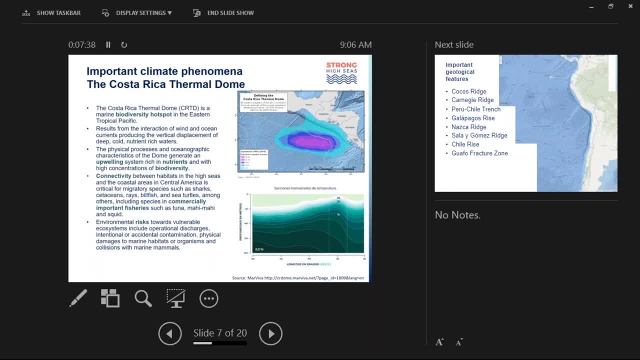 many of these species are very important in a commercial manner of speaking, such as tuna, mahi-mahi and squids. This is an area that has a lot of traffic of ships and commercial ships, and so the environmental risks are very high in this region for collision and oil spills, for example- for the biodiversity. 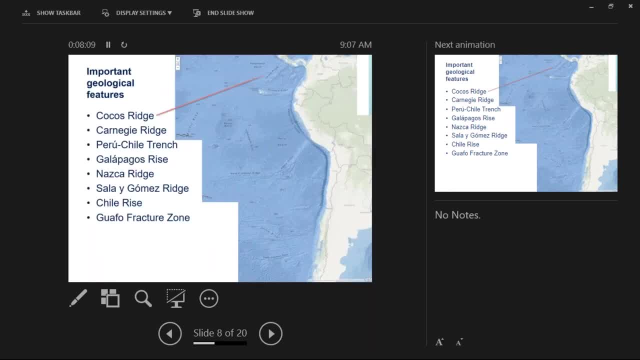 of this particular region. So there are also very important geological features that are associated with the active tectonic framework of the region. We have the Cocos Ridge, the Carnegie Ridge, the Peru-Chile Trench, the La Pagos Ridge, Nazca Ridge, Salay-Gomez Ridge. 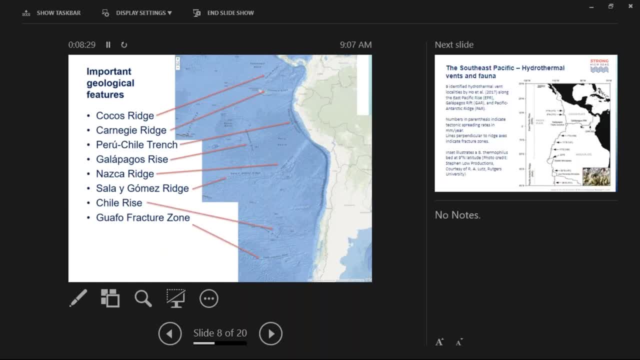 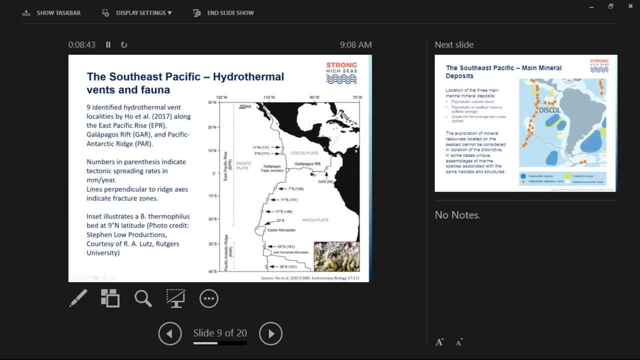 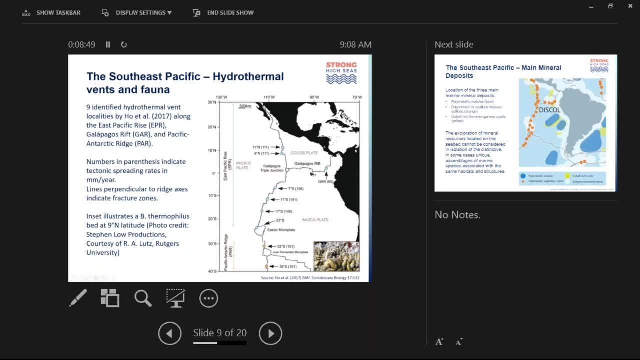 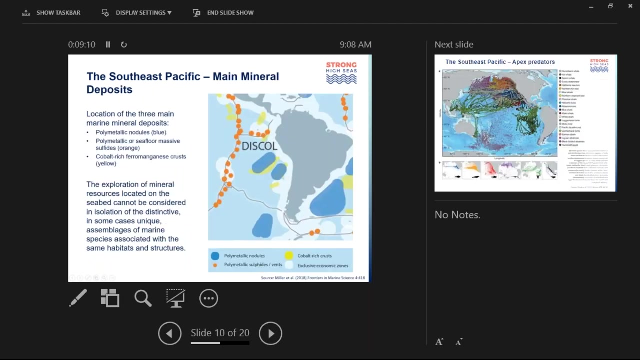 Discover, Well, not discovered. They gathered information on these parts that hold these hydrotelmal parents. there have been 995 hydrotelmal vents along the eastern Pacific rise, the Galapagos Rift and the Pacific Antarctic Bridge. I'm sorry for my English and I apologize. And also it is a region very, With very. 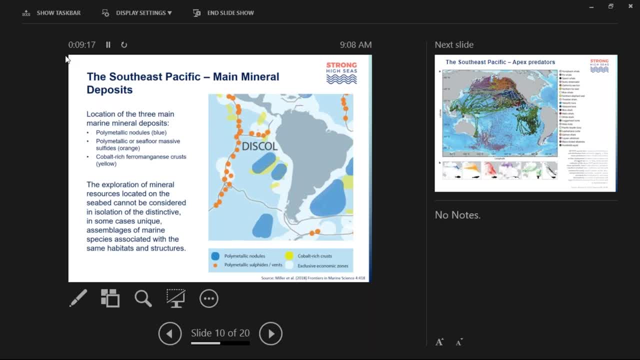 important ставats and馈 zurith 😪. mineral deposits, mostly polymetallic nodules, polymetallic or seafloor massive sulfites and cobalt-rich ferromagnetic crusts. However, it is very important that the exploration of these mineral resources cannot be considered. 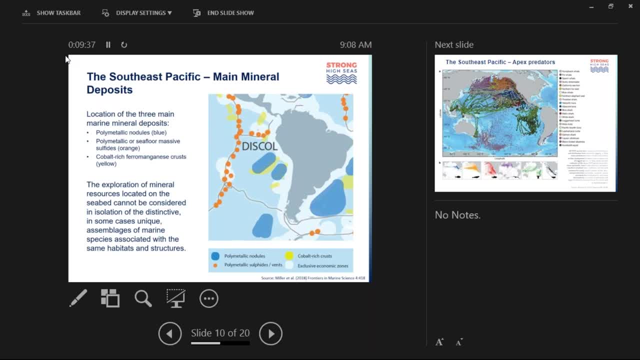 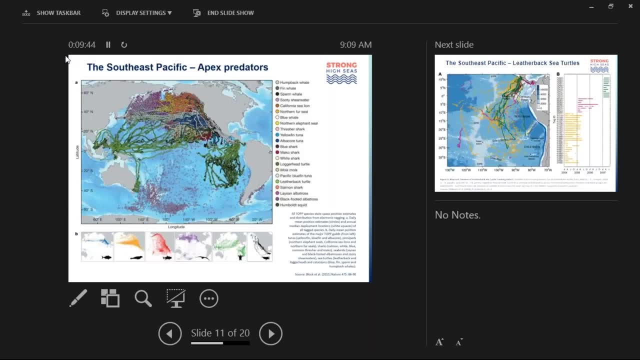 in isolation of the distinctive and, in some cases, very unique assemblages of marine species that are associated with these habitats and these structures. So this region, the southeastern Pacific region, is very important for apex predators. However, we do find that there are a lot of data gaps and information gaps in this region. 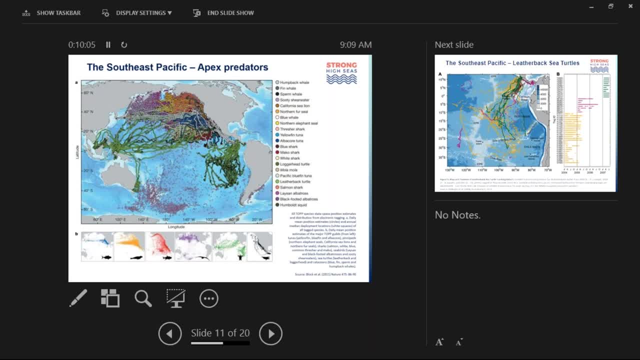 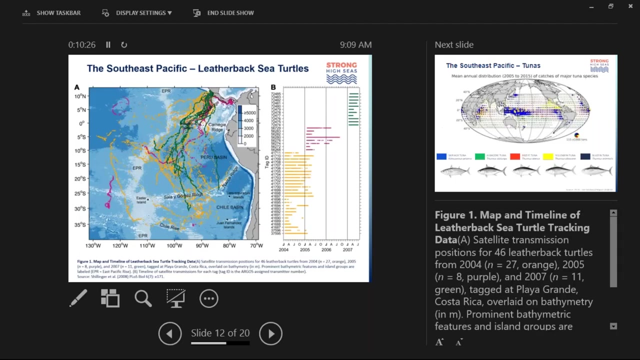 comparing to the northern, the northeastern Pacific region, because the sampling effort has been graded in these regions. But with the information we have so far, we can see that it is a very important migration route for leatherback turtles and humpback whales, among other species. 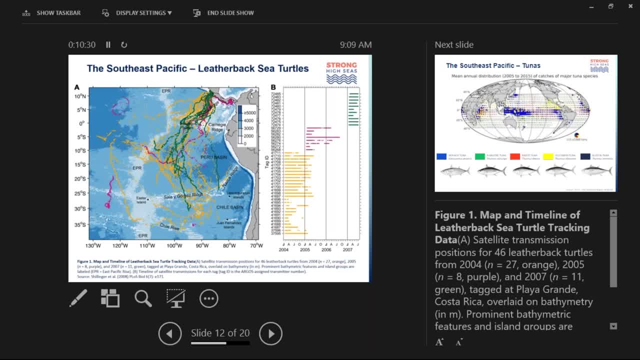 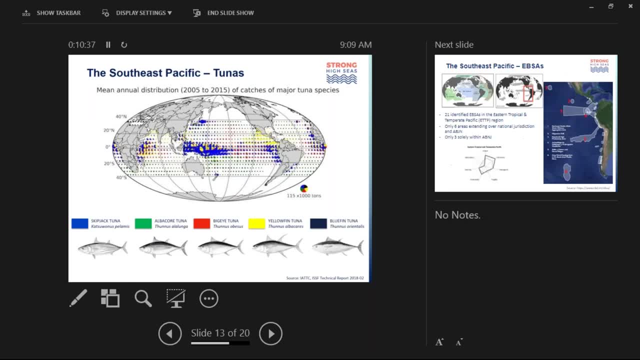 We have also information on leatherback sea turtles, seeing that they can perform migrations greater than 4,000 kilometers, And, in a commercially aspect, we can see that in the In the region, the most fished species are the spikyak tuna and the yellowfin tuna. 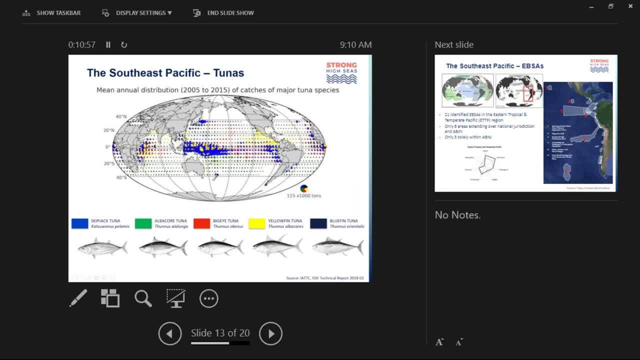 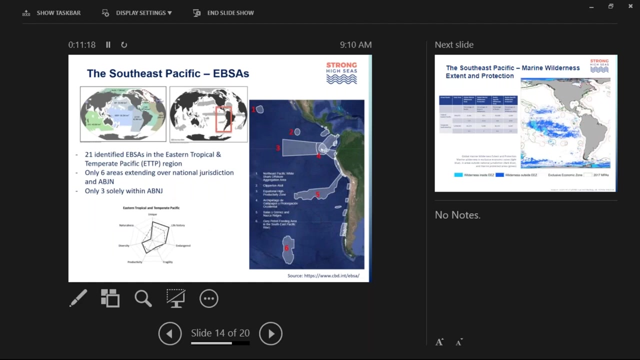 We can see that the spikyak tuna it's more important. the biomass is greater in the south hemisphere, whereas in the northern hemisphere part of the region the yellowfin tuna is greater And And And, as Patrick was telling us before, there are currently these areas being determined. 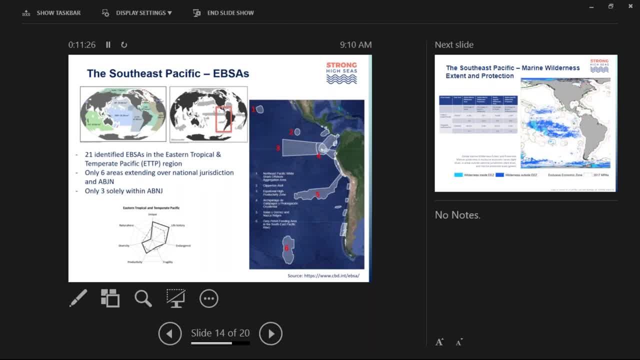 called EPSAs, which are important areas for biodiversity and ecological conservation. So in our area there are a total of 25 identified EPSAs in the well, in the classification of the CBD Covered by the EPSA And Covering the eastern tropical and the temperate Pacific regions. 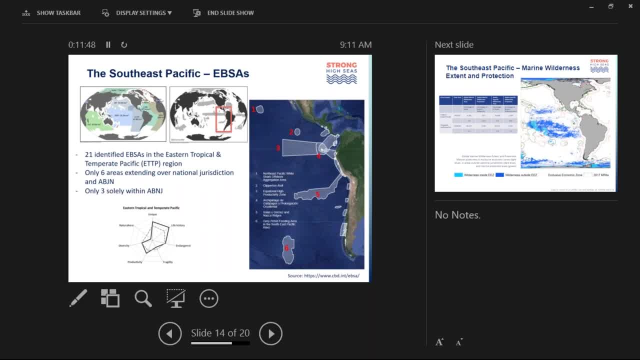 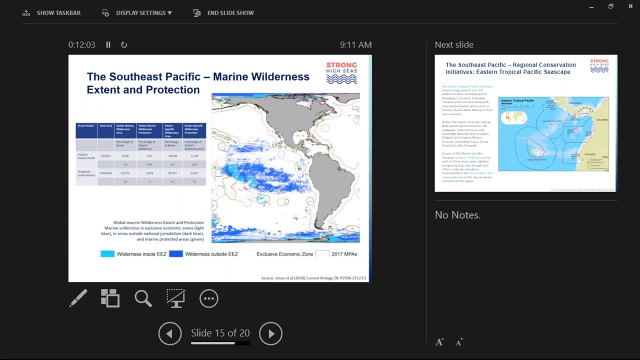 However, only six areas extend over the national jurisdictions into A, B and J And only three are solely located within the A, B and J. So the This is This slide shows These areas in blue that you can see here are areas that have a lower 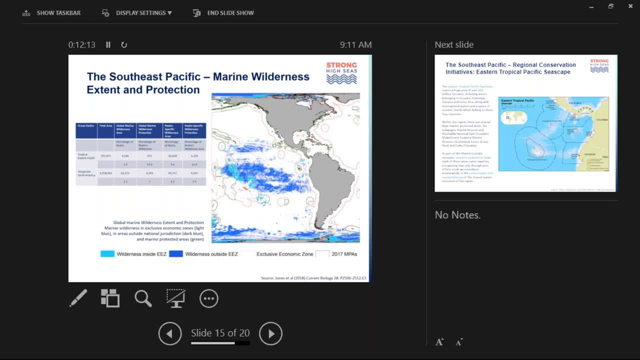 Low Start here. You cannot a lower incidence of human stress factors. And, as we can see, this also shows which – these areas that are within the economic exclusive zones and within marine protected areas, And only about 20 percent of the percentage of the realm within these wilderness areas. 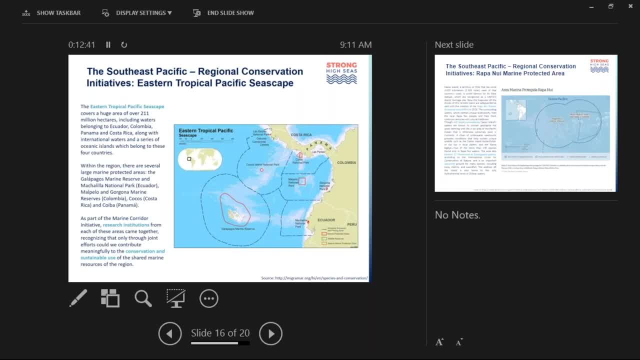 is protected by marine protected areas. However, there are some initiatives for the conservation in ABNJ areas And we have, for example, the Eastern Tropical Pacific Seascape, which is a corridor between the Kalapagos Marine Reserve, the Cocos National Park, Coiba National Park in Panama and Malpelo. 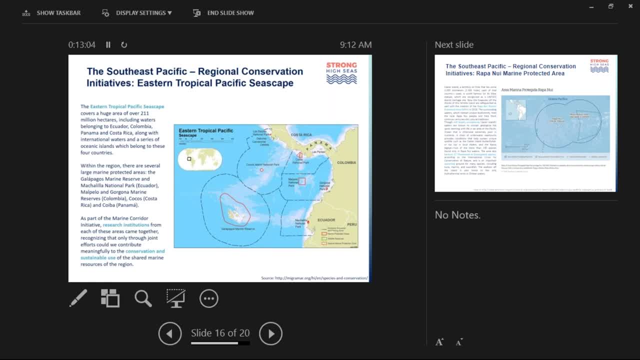 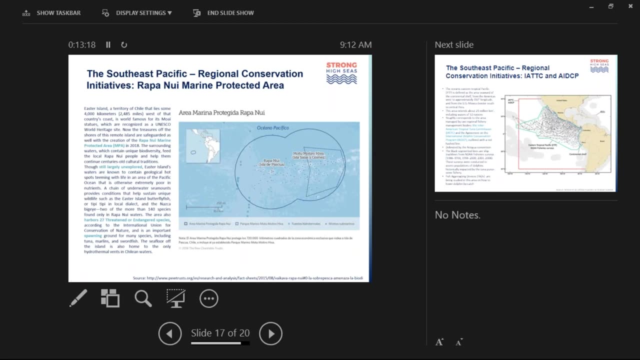 and Gorgona National Parks in Colombia. There are some other protected areas that are located in coastal regions, such as the Machalilla National Park, Las Baulas, Sostenal, Camarones and Caletas. Also in the region, Chile has been developing a lot of marine protected areas in the last 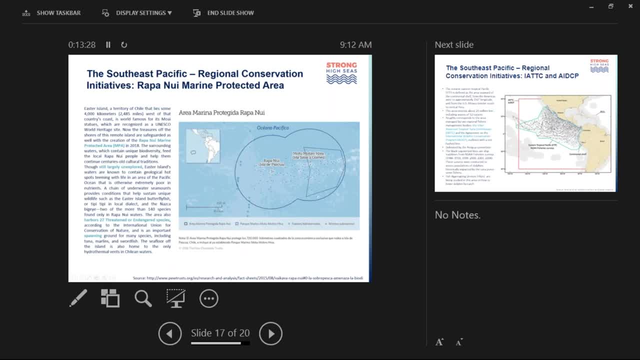 few years And we have here an area that is being declared in the Eastern Island Protected Area, And this is also very important, Because it is – it's very important. This is a region that is in the migratory path of many, many species as well, and is 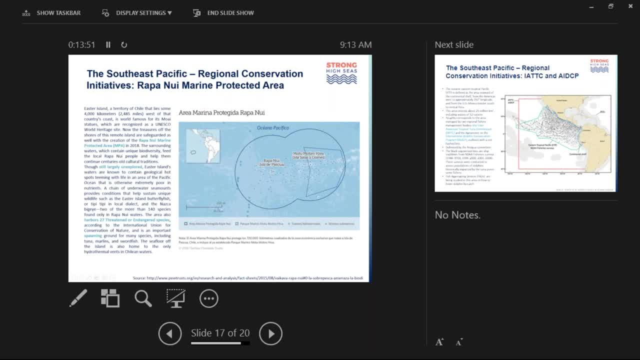 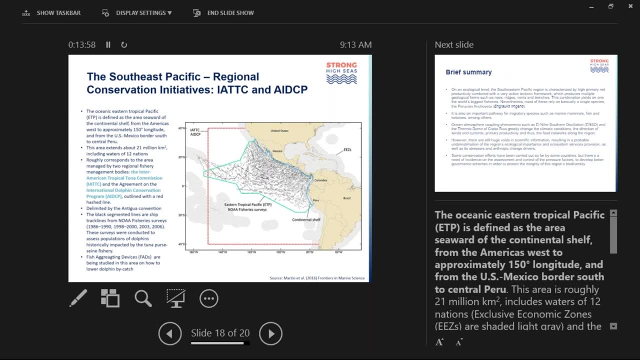 very important for commercial fishing, although it is still largely unexplored. And also the Inter-America Tropical Tunic Commission and the International Dolphin Conservations have been performing many – well many- experiments with fish aggregating devices, So the dolphin and other important species and endangered species bycatch are lowered. 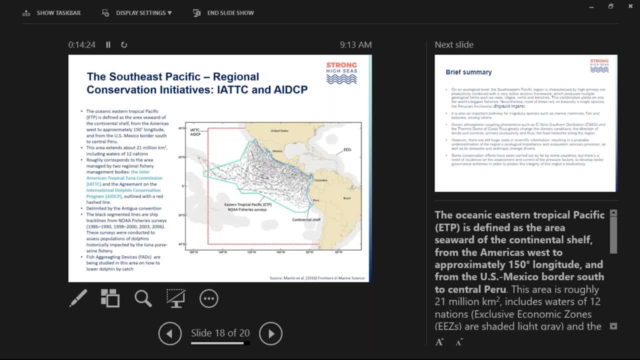 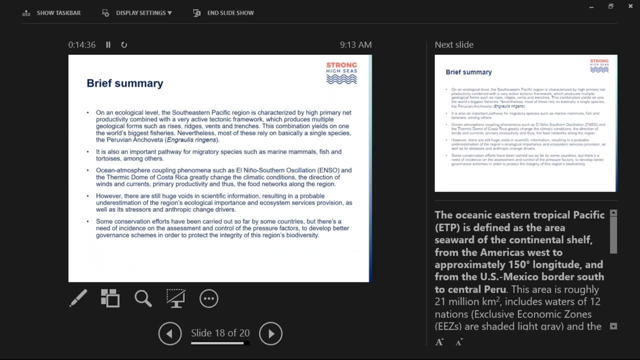 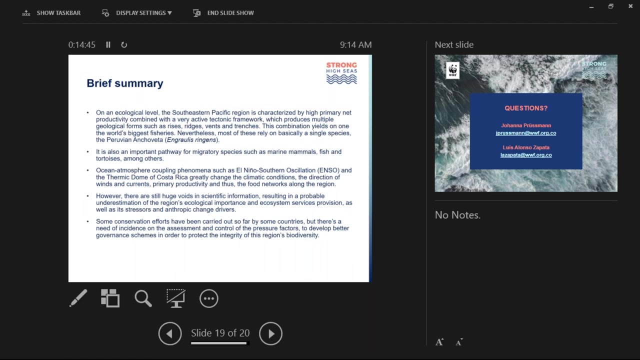 using these devices that allow to aggregate different kinds of species and trying to develop techniques that avoid the bycatch of these other important species. So that's it, Thank you, Thank you, Okay. So, to summarize, on an ecological level, the Southeastern Pacific region is characterized. 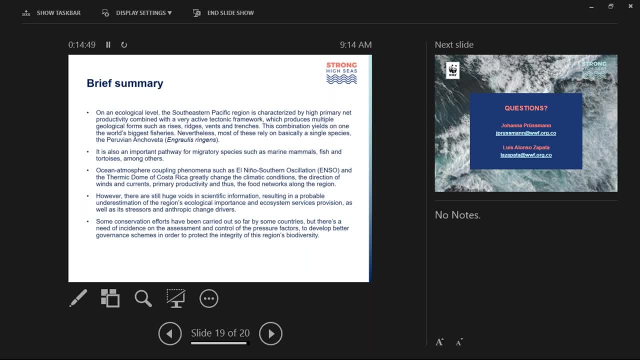 by high primary net productivity, which is combined with a very active framework which produces multiple geological forms, such as rises, ridges and trenches, And this combination yields on one of the world's biggest fisheries. However, most of these rely on basically a single species, which is the Peruvian anchoveta. 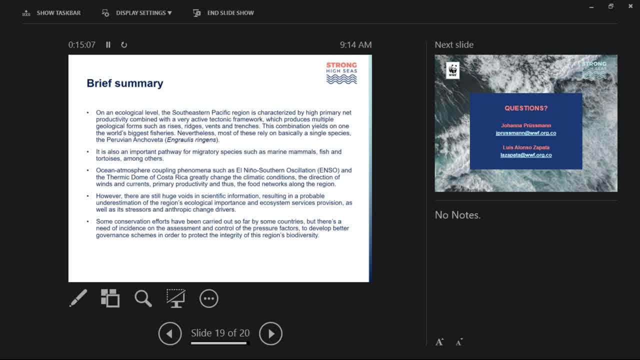 It is also an important pathway for migratory species. So some marine mammals, fish and tortoises and tortoises, among others. The ocean-atmosphere coupling phenomena such as the ENSO and the Thermic Dome of Costa Rica greatly changed the climatic conditions, the direction and the 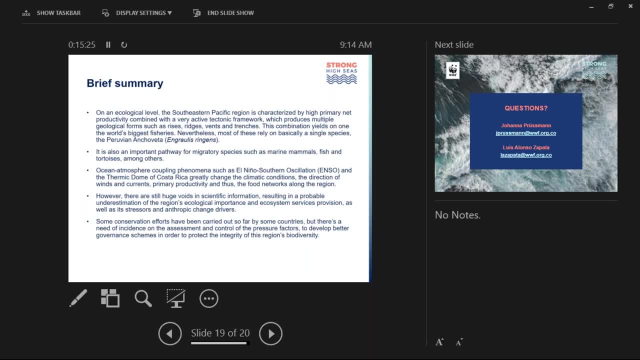 productivity and thus the food networks along the region. Nevertheless, there are still huge voids in scientific information, resulting in a problem in the estimation of the region's ecological importance and the ecosystem services that they provide, as well as the stressors and 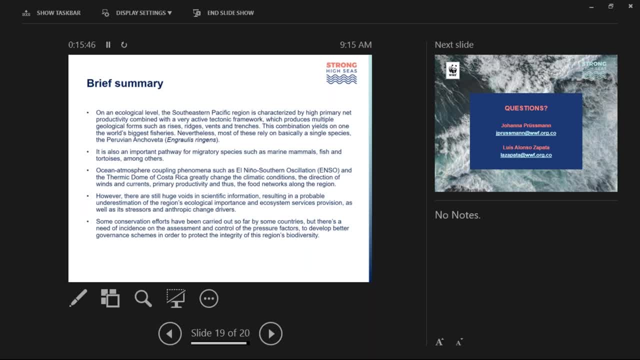 the anthropic change drivers. But some conservation efforts have been carried out so far by many countries, but there's a need of an incidence on the assessment and control of these pressure factors to develop better governance schemes in order to protect the integrity of these regions'. 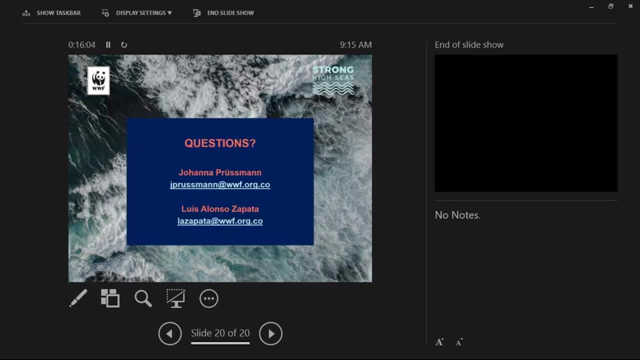 biodiversity. So, if you have, If you have any questions, we can answer afterwards during the Q&A session and also you can email us with any questions or information that you may need. Thank you very much. Thank you, Johanna, for a great presentation. We had a few questions come in, so excellent. 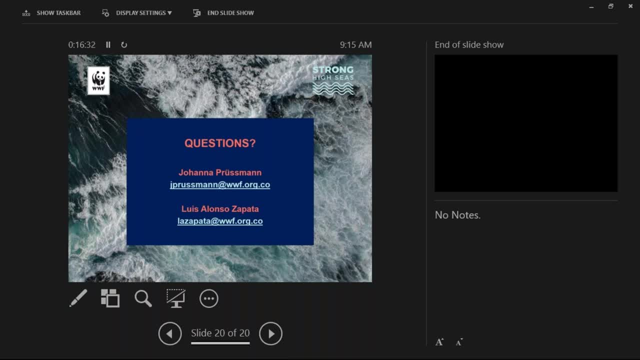 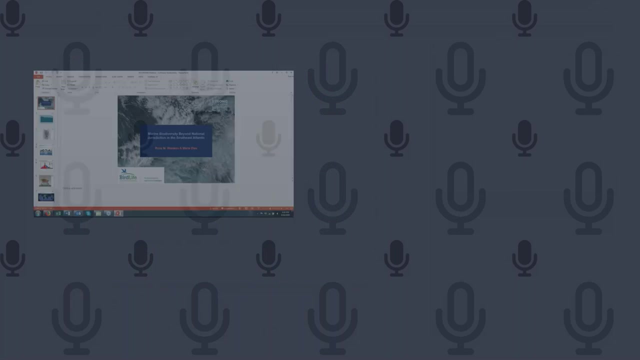 We will come back to the questions now, after the next presentation, But please feel free to. Please feel free to write more questions into the box on the side and we will get to them in the next Q&A session. Now we're going to hear a presentation from Ross Wanless, from. 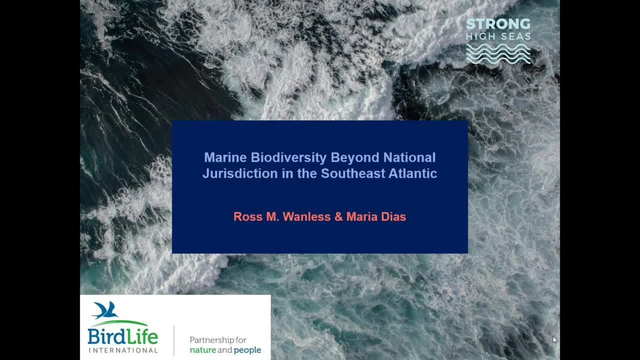 BirdLife International Africa, focusing on the Southeast Atlantic. So please, Ross, Can everybody hear me? Yeah, I think I can. Yeah, I think I can, Yeah, I think I can. Yes. Now, loud and clear, Ross, please go ahead. 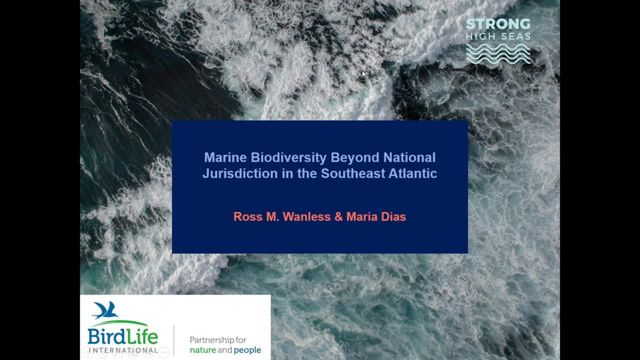 Okay, Great, Hi everybody, Thanks for that, And I'm going to be taking a slightly different tack from Joanna in that I will be presenting a slightly broader overview of marine biodiversity, some of the threats and pressures, looking at some of the connectivity things that Patrick touched on as well and making a case for 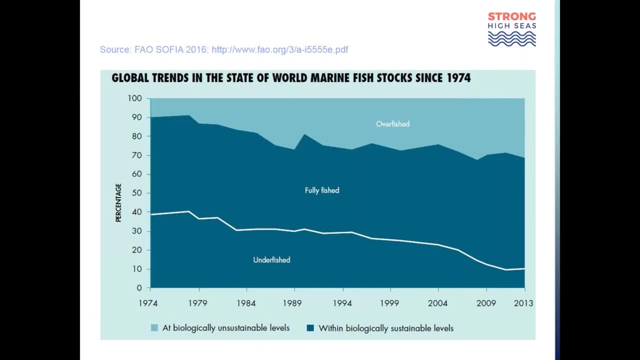 the need for biodiversity conservation and spatial conservation in the high seas. This talk was prepared with support from Maria Diaz, my colleague from Cambridge. Okay, So the number one impact that human beings have on the ocean by a very long yard, and not just the ocean, on its ecosystems and the biodiversity in the oceans, is, of course, fishing. 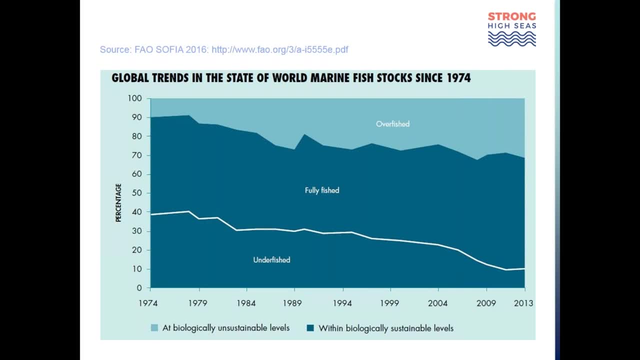 The Food and Agriculture Organization, or FAO, is a very important organization in the world and we're able to apply this to our products, to the marine biodiversity, marine lives and, as you can see, they're constantly changing, And we're taking a look at aircrafts and we're taking a look at products produced. 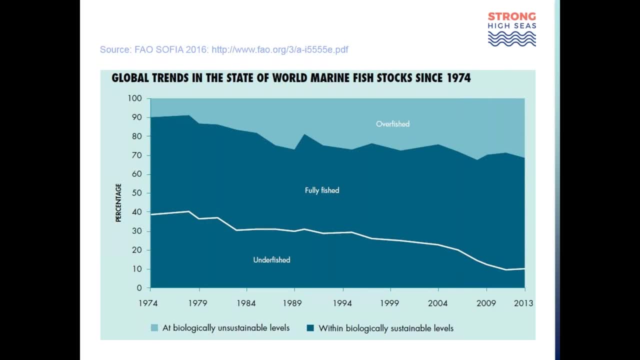 by the NAO. this is, by the way, an example of an aircrafts market, So the world's most annual state of the world's fisheries report from 2016.. I've taken a screen grab from that And you can see. the key point of interest on this graph is the light blue section at 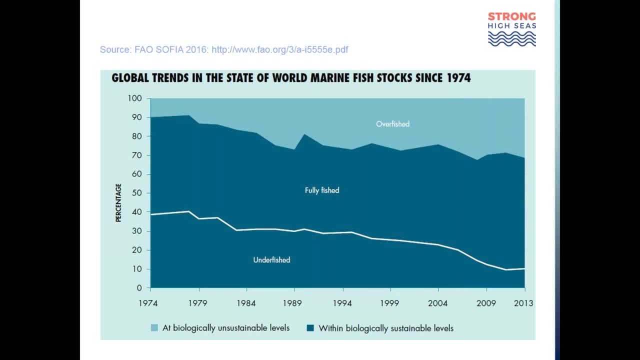 the top And you can see there's a downward trend from around 90% of stocks were fully fished or under fished, which is the state that, according to FAO, you want to be and you want to have your stocks fully fished. 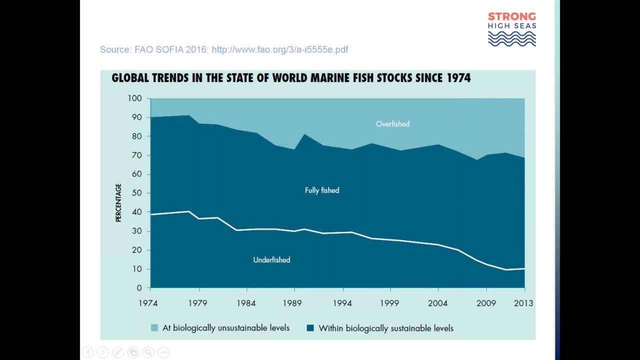 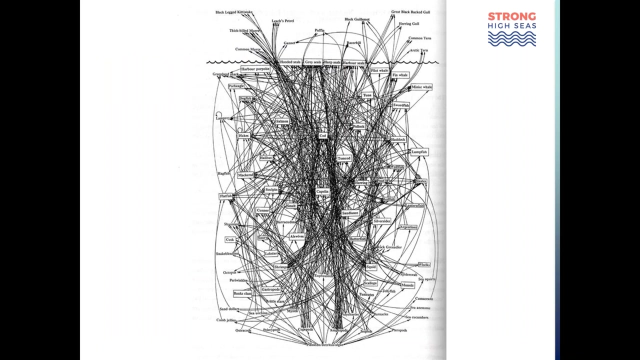 that means we're maximizing the production of protein from the ocean, and that's declined to about 75% in more recent years. So, sadly, we are now able to extract considerably less protein from the oceans than we were previously. The interconnectedness of marine food webs makes it very clear that we can't 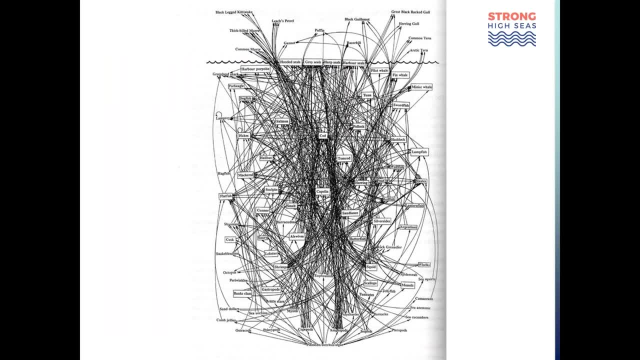 simply remove vast quantities of a certain species and be certain that the ecosystem will continue to bounce back or function the way it used to. What you see on the screen here is a scribble diagram listing 50 or so species and the various relationships between them. As you can imagine, 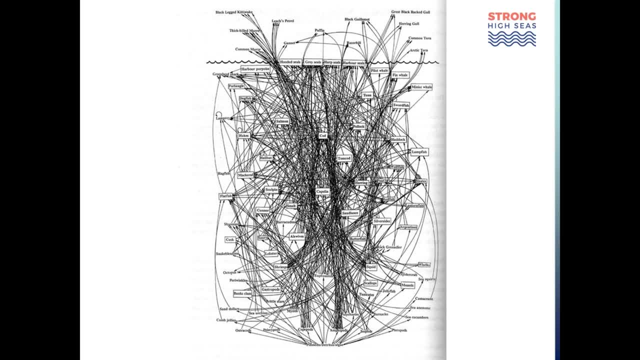 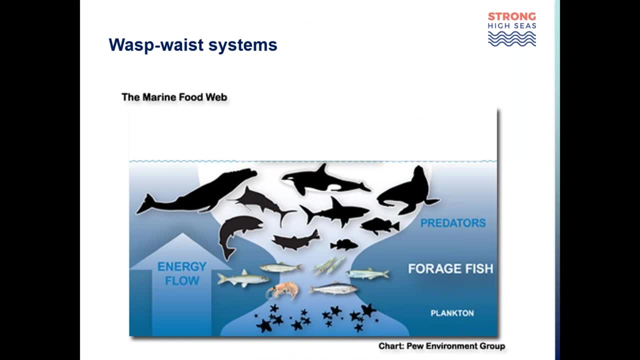 you pull out one species from that system or vastly reduce the numbers of individuals in that species. So if you look at this graph, you can see that there are about 50 species from that system and it's going to have some fairly profound effects. 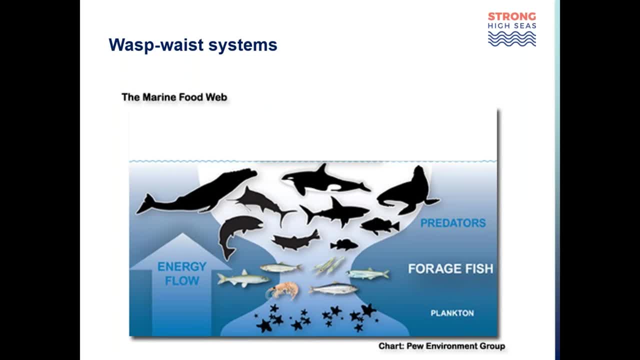 I'm going to drill down a little bit now into the upwelling systems- and Joanna touched on these previously- but just to give a little bit more detail, these are classic wasp waste systems. In other words, there's a huge biomass and diversity of predators at the top of the food. 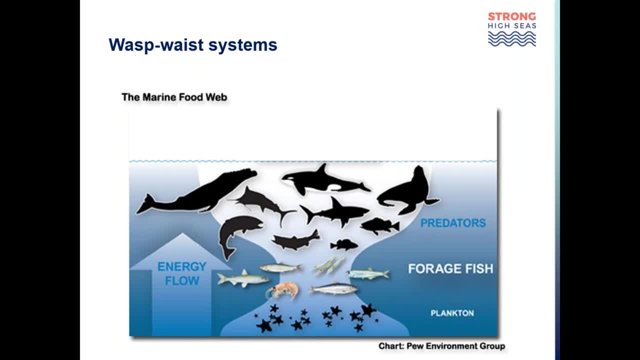 chain. There's a huge diversity of plankton and smaller organisms, but those tend to be funneled through a very few species in the middle. Those are typically the anchovies or sardines and those are heavily fished. Those are called forage fish. 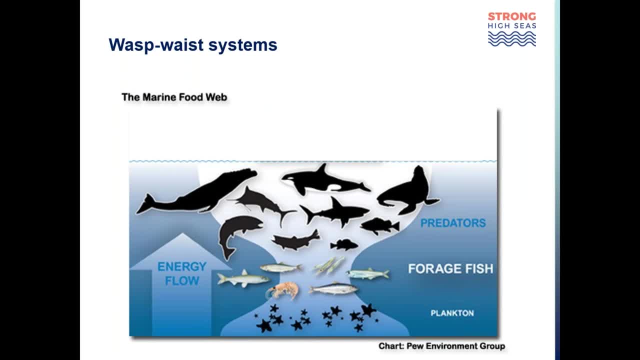 because everything eats them, or everything eats the things that eat them. Tackling forage fisheries is the new frontier in terms of sustainable ocean management. We really have some gigantic challenges ahead of us if we start taking out the krill in Antarctica or the anchoveta in the Pacific or the sardines in 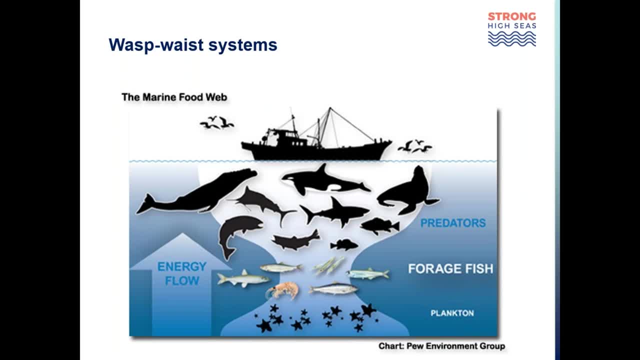 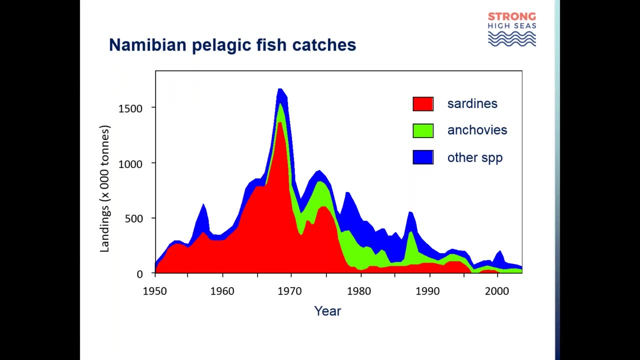 the Benguela. In fact I'm going to show that to you now. an example of Namibian pelagic fish catchers You can see in the 1960s and early 1970s- the red is the sardine- rampant overfishing of the sardine stocks. In peak they were taking almost 1.5 million tons. 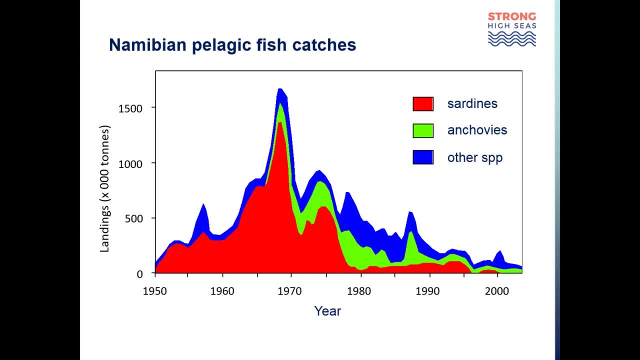 of sardine a year. Huge collapses, a bit of a switch to anchovy. further collapses, and so it went on up until 2001, when the last sardine was caught in Namibia. The sardine has been caught in Namibia since then. 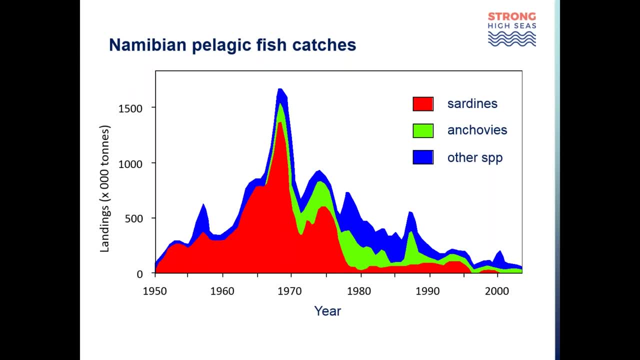 Nothing, and not a single sardine, has been caught in Namibia since then. Look what happens when I overlay the population numbers of African penguins, which are specialists on anchovy and sardine. The scale is on the right-hand side. It's a completely different scale. 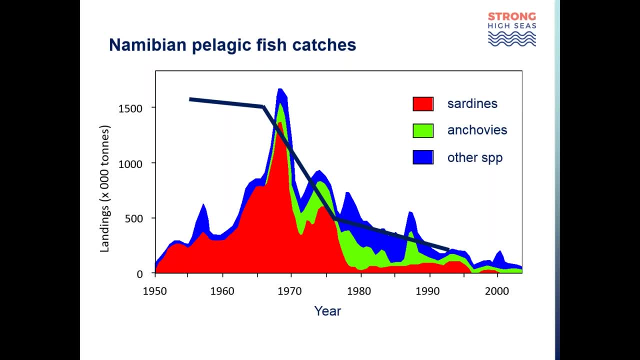 so we're not talking about 1.5 million tons of sardines, It's a completely different scale. so we're not talking about 1.5 million tons of sardines, It's a completely different scale. so we're not talking about 1.5 million tons of penguins. 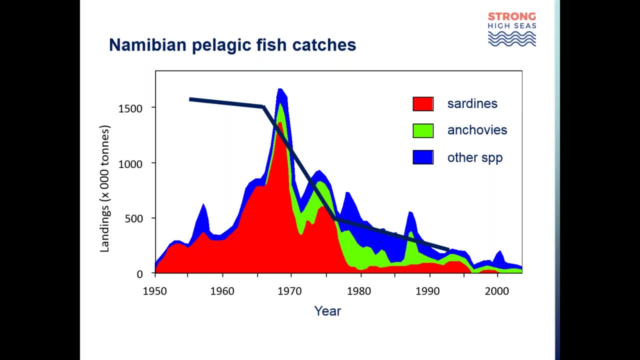 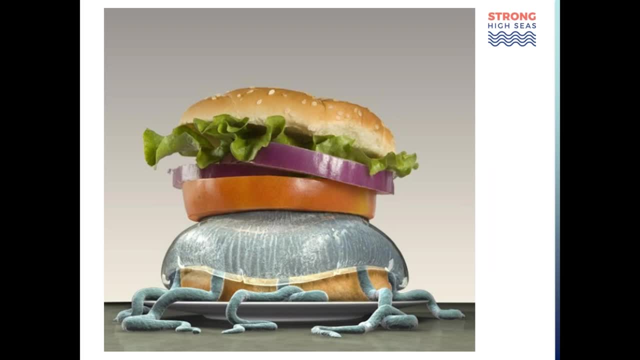 So don't get confused by that, but it's just an illustrative thing. I hope you can see that that downward trend, that crash, matches very, very closely with the rampant overfishing and collapse of the stocks, And so we seem to be heading to a changed ecosystem, The point I was making earlier. 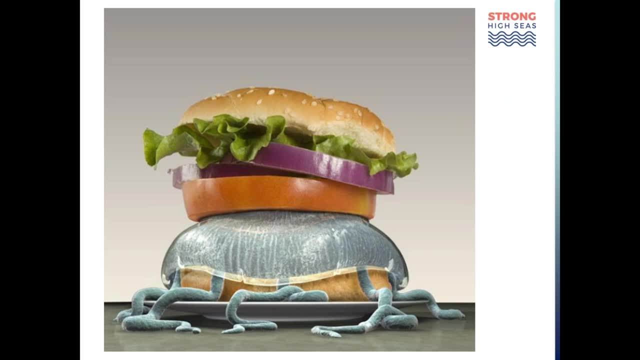 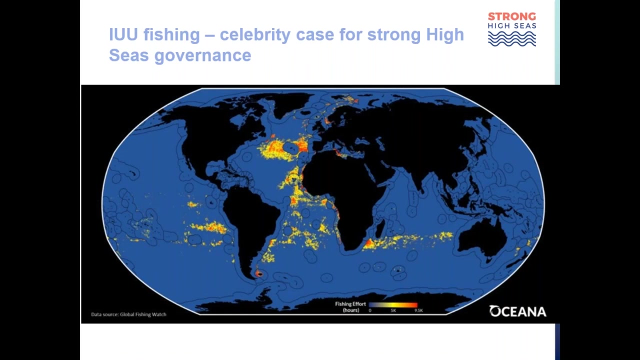 Namibia's ecosystem is now dominated by jellyfish or gelatinous species, and these things consume small fish, which makes it really, really unlikely that the Namibian ecosystem will ever be able to recover to its former fish-dominated state, And so, indeed, perhaps we will be enjoying jellyfish burgers from Namibia. 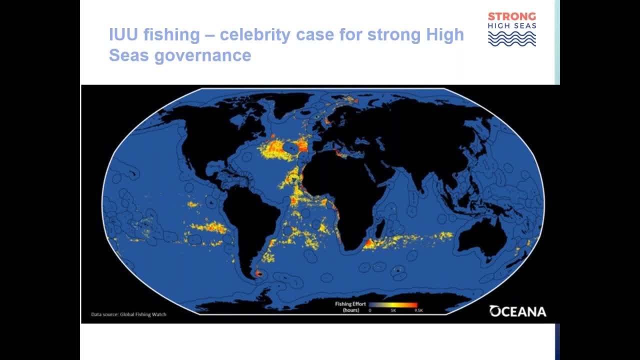 before too long. The impact of fishing is obviously pervasive and it's the number one we face to conserve ocean biodiversity. And it's all good and well setting rules, but illegal, unregulated and unreported fishing is a gigantic challenge And this is a heat map. 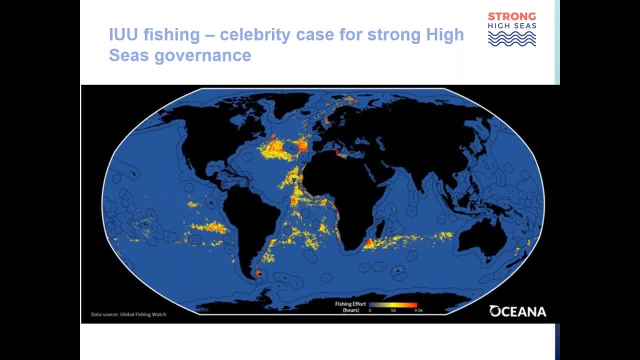 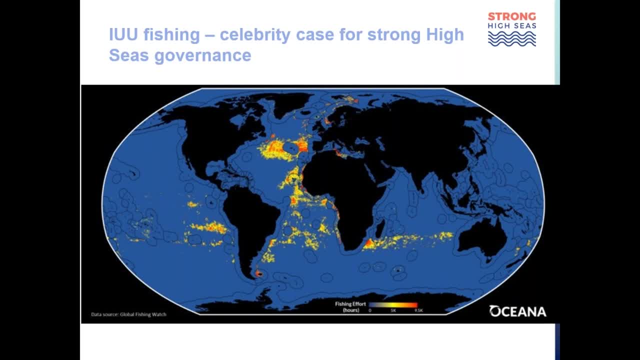 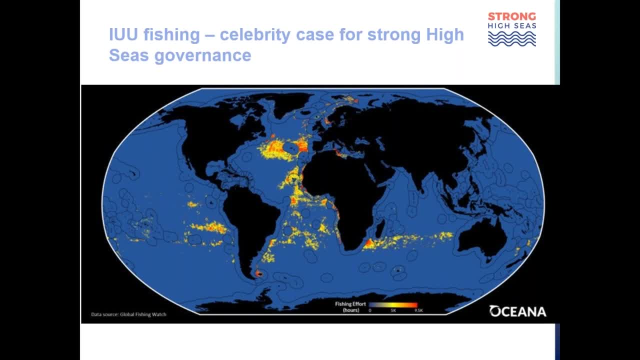 abiding fleets, not exclusively. There are some challenges there, But I'm using this to illustrate just how widespread fishing effort from certain nations is And if you can consider the scale of the ocean, how difficult is it to know which vessel is fishing exactly, where and when And how. 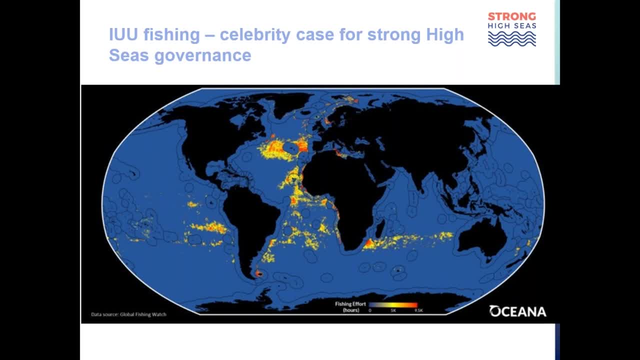 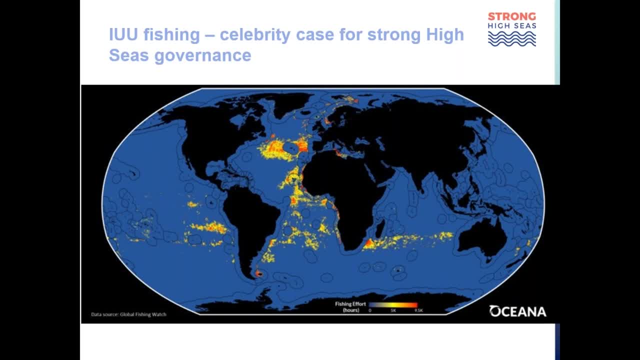 in countries to manage fishing impacts, because it's not reported, We don't know where the fishing effort took place, how many fish or what species were caught, what gears they were using even, and so you can't manage impact, you can't manage sustainability. if you have widespread IUU fishing, This is going to 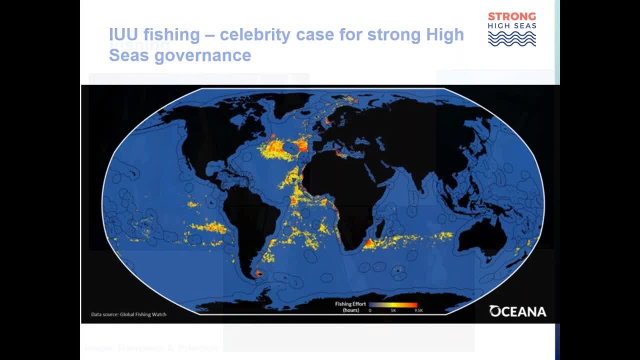 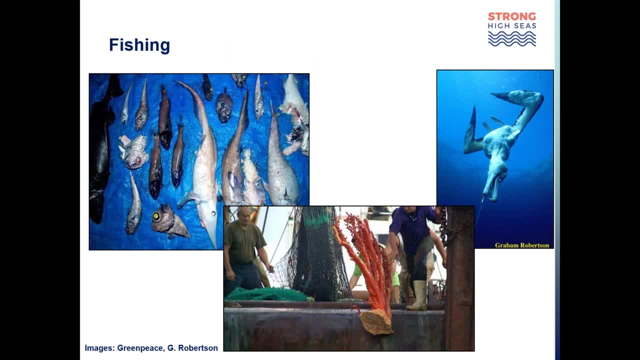 be one of the challenges that humanity is going to have to grapple with in the in the very near future. A talk on fishing wouldn't be complete without mentioning the non-target impacts, or bycatch, incidental capture, and this is a huge focus for BirdLife International: solving problems of seabird bycatch. but 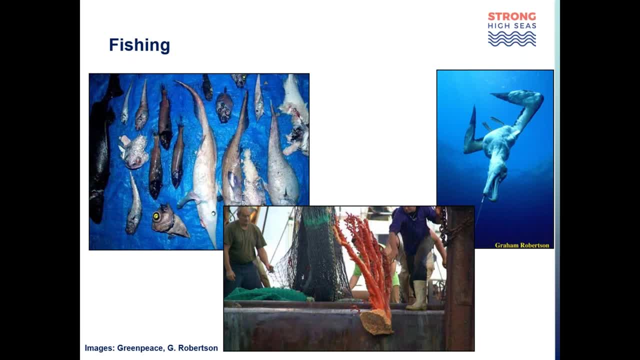 the incidental capture of other species continues and is hugely problematic around the world. These are the species which are typically discarded as dead. they have no commercial value and yet they can cause the collapse of species, of the bycatch species, without causing the collapse of the target species. So we have a 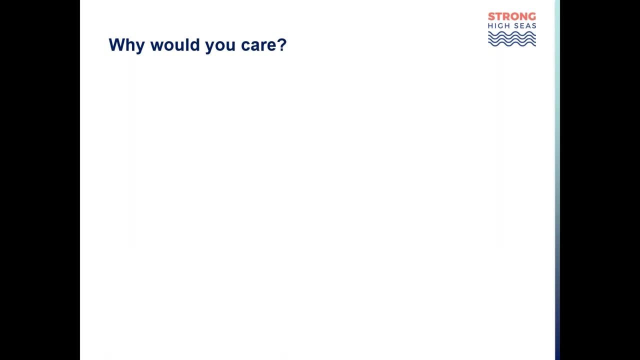 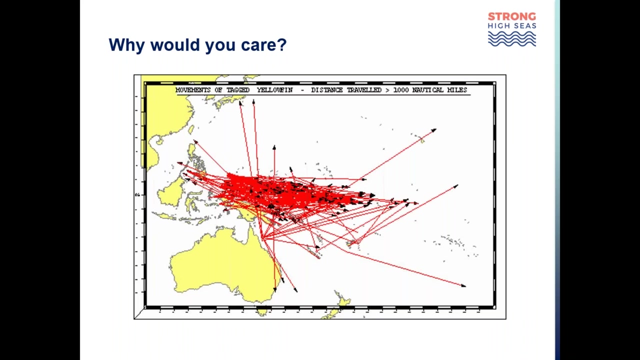 bit of a problem there that we really need to solve, and many people are working really hard to find ways to catch fish sustainably without causing non-target impacts. Now why would you care about this? Why do you care about what's happening in the high seas? And Patrick certainly alluded to that, and so 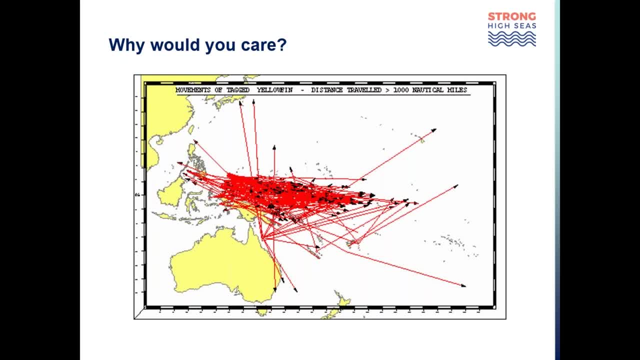 did Joanna. Here's another lovely image of a tuna tagging program and you can see that the concentration of where the fish were caught is right in the center. but some of those tuna that were tagged in this program moved massive distances and the connectivity from a country's exclusive economic zone into the high seas is. 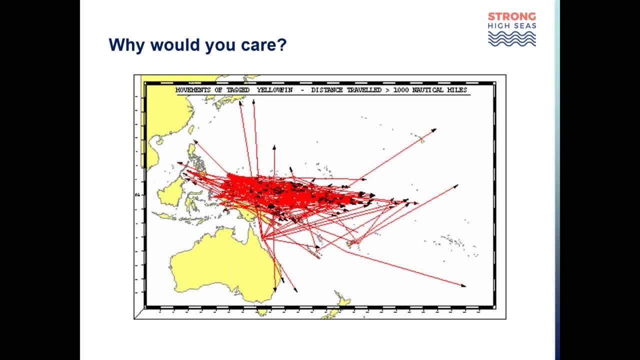 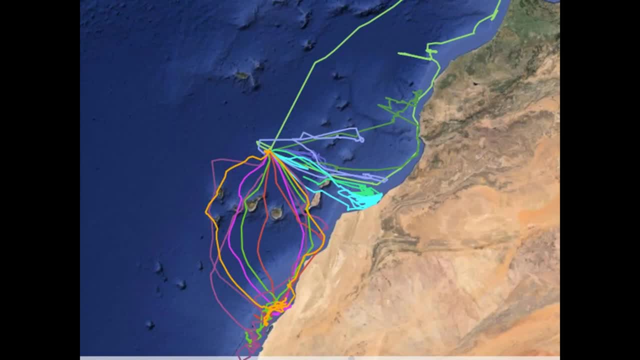 everywhere in the oceans. Oceans operate fundamentally differently from how landscapes and terrestrial environments operate, and that connectivity is difficult for us as humans, which are very terrestrial species, to get our heads around. Here's another example of some really impressive connectivity. Moving on to seabirds, we can see that you've got a species of shearwater. 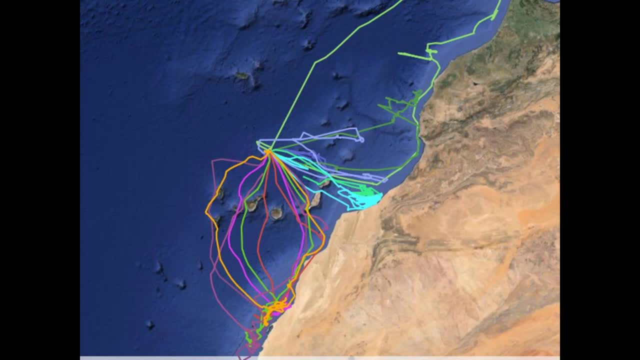 breeding on an island, but all of its- and this is off the coast of Africa. all of the foraging is being done along the shoreline of Africa, and so these birds are moving from one country through the high seas into another country, and if they're caught in that second country, whose responsibility is it Another? 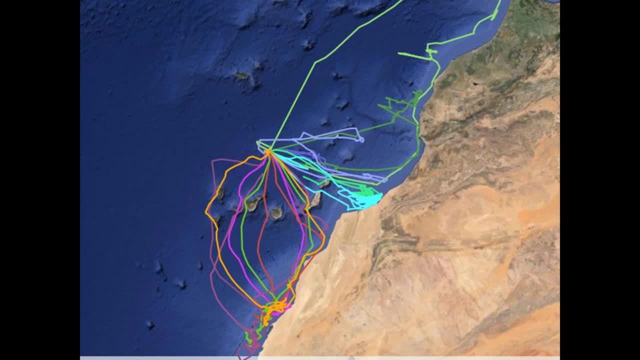 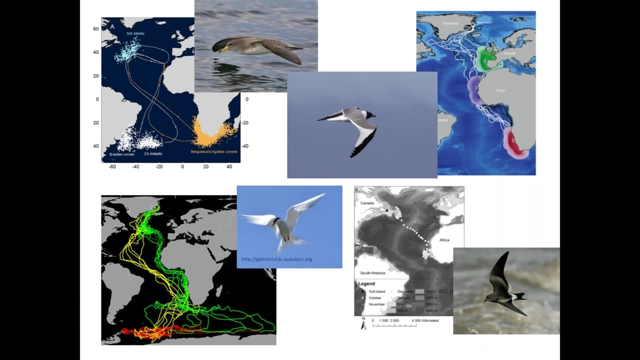 question to ask is: whose bird is it? If it is caught in your waters, is it your bird and your problem, But if it breathes in another country, is it their bird and their problem? Seabirds are, of course, highly visible, and they're cheaper and easier to study than many other marine. 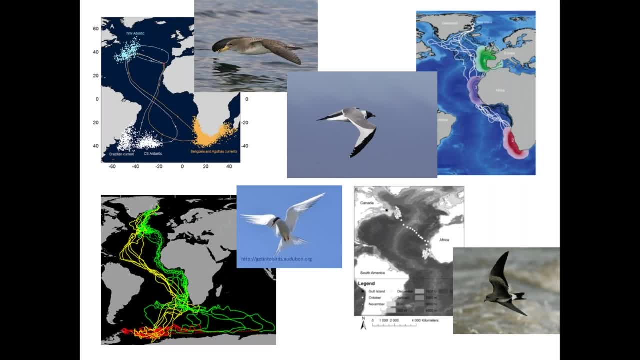 species and seabirds demonstrate how massively interconnected the Atlantic Ocean really is, and you can see from just these four examples of how widely animals these seabirds move across the Atlantic Ocean and the diversity of migratory patterns that they show. Some hug the Eastern Atlantic seaboard. 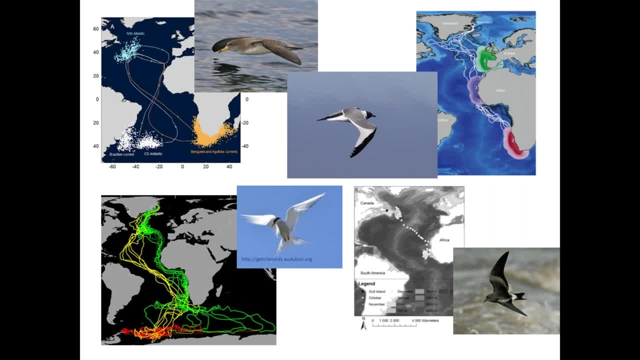 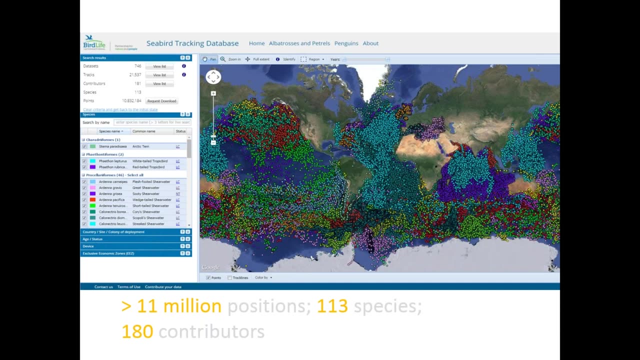 others crisscross the Atlantic Ocean, some move just minor distances. There's a huge range of strategies and processes at play here, and so we've really got to think big if we're going to tackle marine conservation for highly migratory species, And it's not just the Atlantic Ocean that has 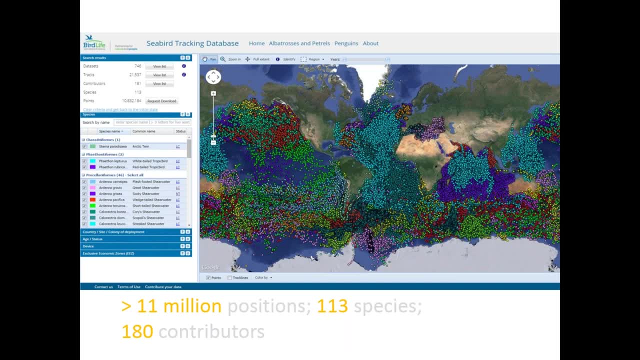 all of this migratory connectivity- and this is a screen grab from BirdLife International's seabird tracking database- and it's clear from this image that there is no part of the ocean that isn't used by seabirds at some point, And so we need to use these data to understand where the hotspots and 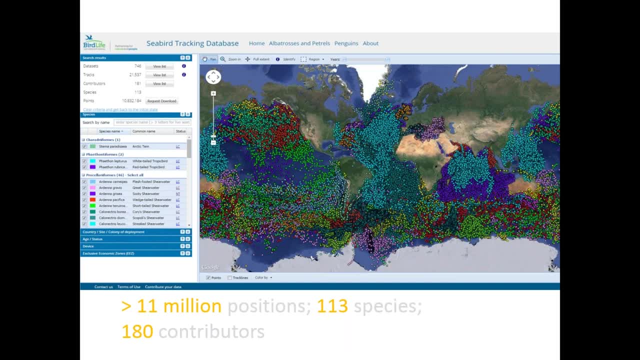 Patrick again alluded to marine important bird areas and how those have been fed into IBSAs and we really need to strengthen those processes and really get turtles and sharks and cetaceans and fish and other things into these sorts of analyses with the sort of tracking data so that we can truly understand. 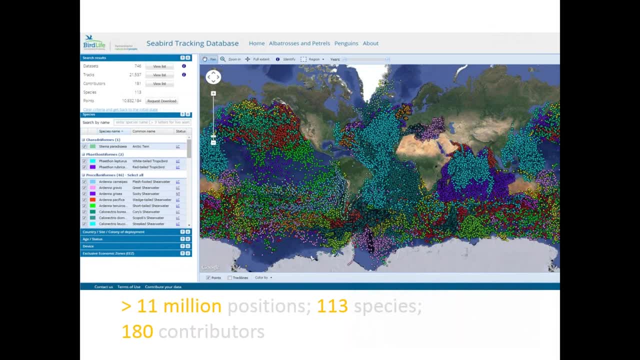 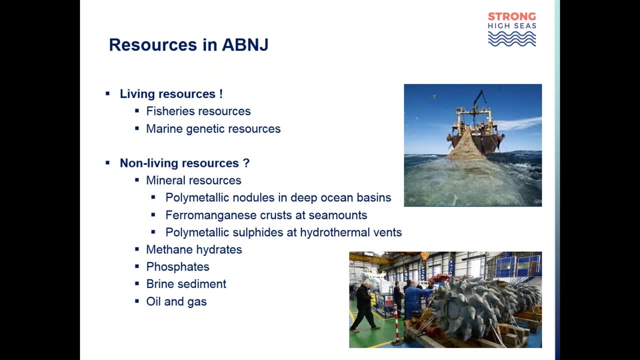 where we're at. Resources in the areas beyond national jurisdiction extend, of course, far beyond just seabirds and just fish. Besides fishing, there are marine genetic resources, and new drugs and new cures for cancer and so forth are probably going to be found from marine organisms as much as anywhere else, because the marine 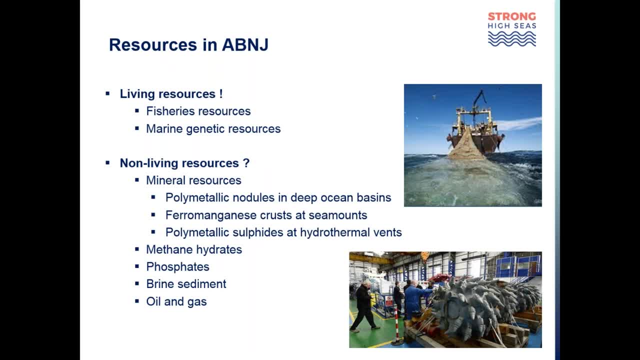 biodiversity is so high And, of course- and Joanna alluded to this- lots of mineral resources, and human beings are starting to access those resources. We're not sure what the consequences of deep sea mining are. We're not sure what the consequences are if you suck out all of the nutrients, such as phosphates and 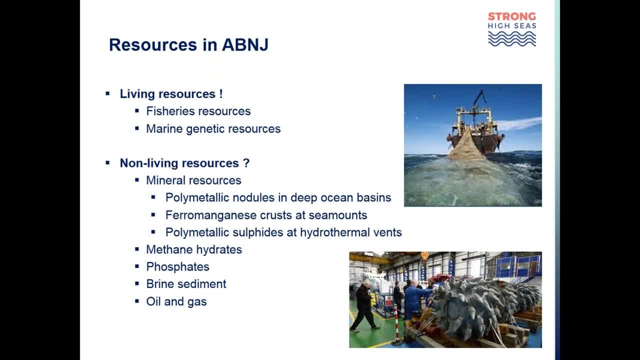 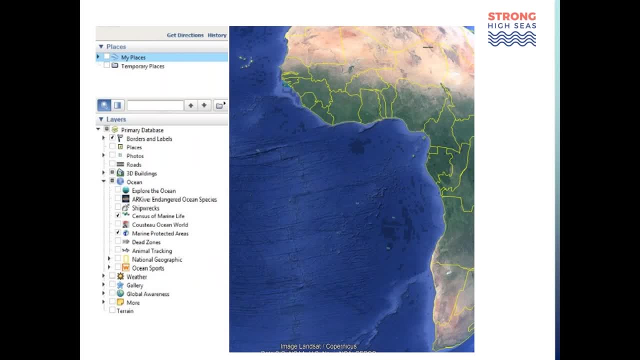 minerals from a seabed. What does that do for the productivity in that ocean, in that area of the ocean? These are big unknowns and we've got to be really careful and conservative about how we go in and deal with the ocean. My closing point is really around productivity and conservation. We know the ocean is full. 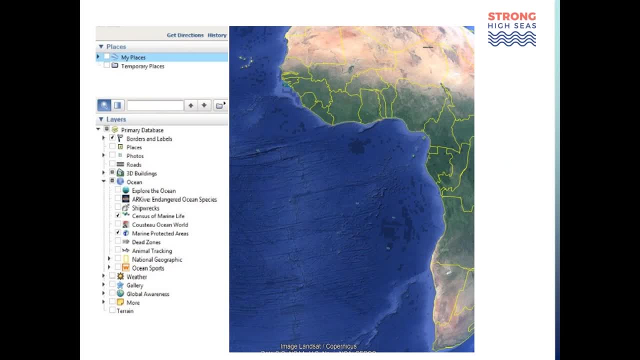 of cool biodiversity, highly interconnected systems, vectored. that connectivity is vectored by birds, whales, fish. It's also vectored by ocean currents, shipping and the so-called distant water fishing fleets. So how are we doing in protecting our oceans? Where are we at And noting that there? 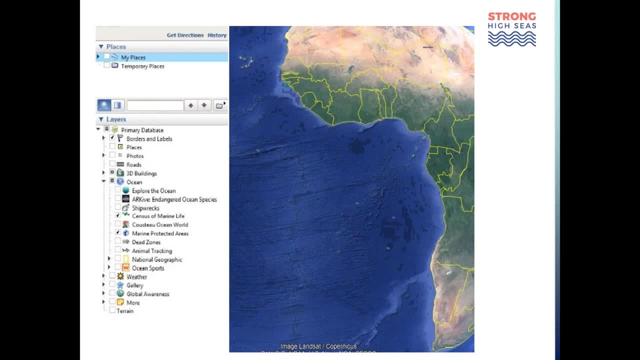 are processes that Patrick mentioned, but those are still very much up in the air and no decisions are out there, and that's what the project that we're part of here, the Strong High Seas Project, is geared. to try and understand What I did here is went on to Google Earth and I clicked on a couple of layers. 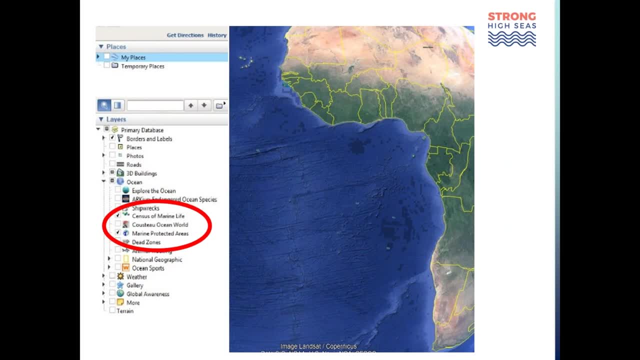 Particularly, I want to draw your attention to the census of marine life and the layer of marine protected areas And, as you can see from the map, it looks startlingly like there's nothing there. In fact, those layers are there. they are. 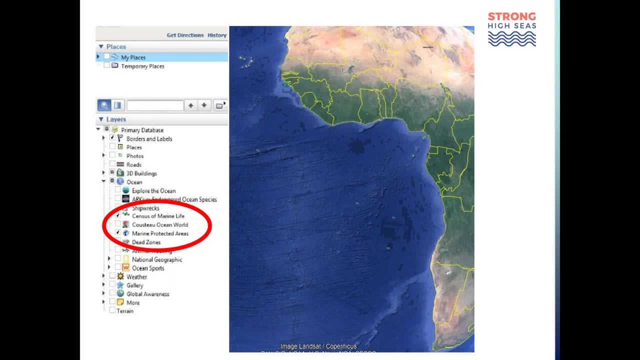 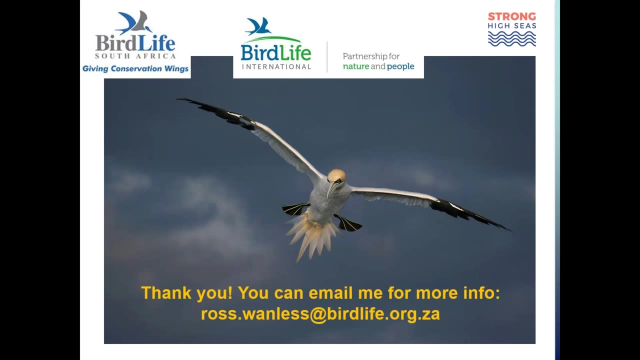 present, but we have so little information about what's out there and we have done so little to protect the ocean environment that it's clear we've got a long way to go And the BB&J negotiations, hopefully, will help us deliver some meaningful gains so that we can protect this incredible. 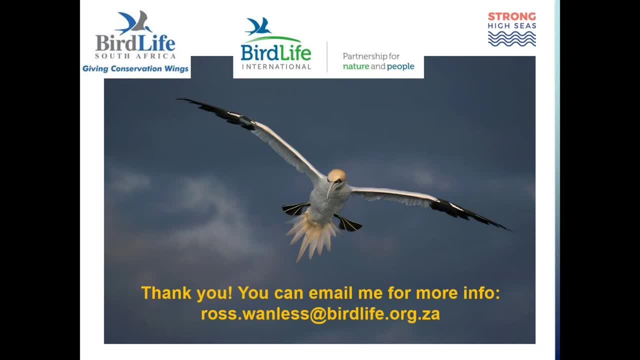 biodiversity upon which so much of our society rests. So thank you very much, and I'm happy to take questions, And there's my email address for those who wish to send me an email. Okay, thanks, Ross, That was a great presentation. 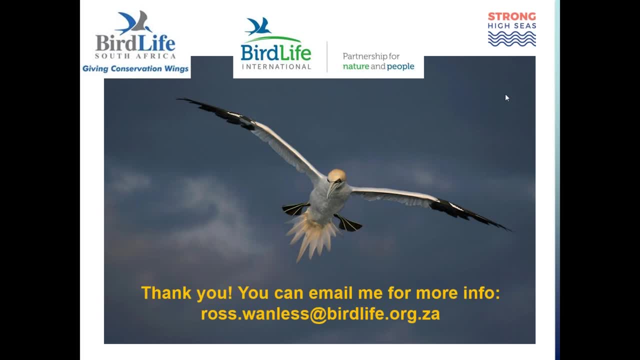 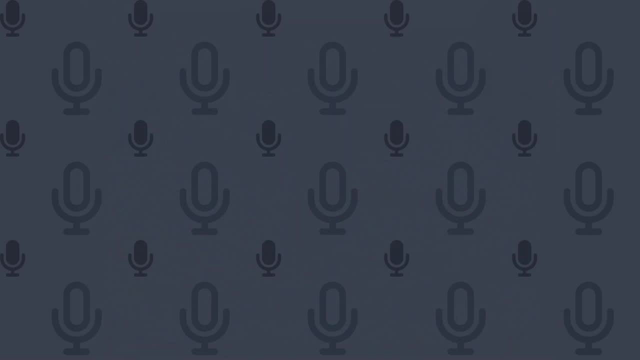 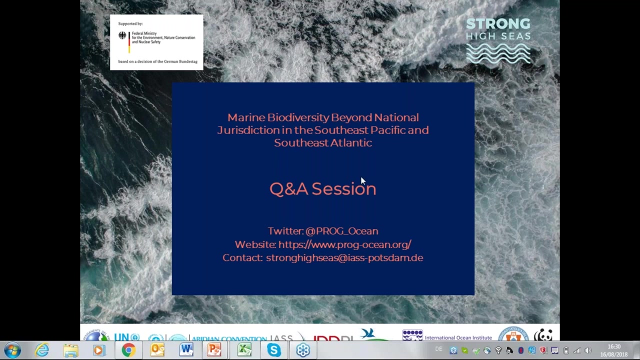 Super interesting. We're now pretty much coming to the end of the hour, as planned, but we had a few questions come in, so we're going to go another five minutes and try to answer at least a few of them for those who want to stick around And 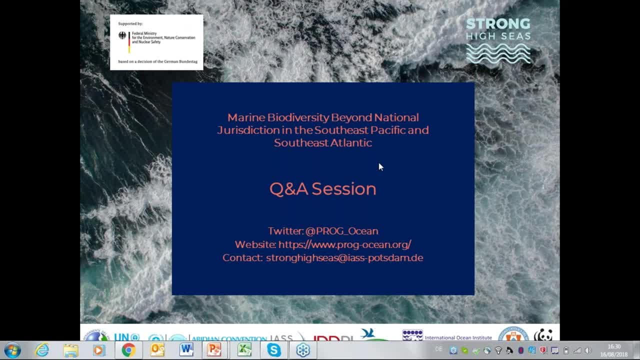 then we'll end it there and I guess any questions that come in we can try to deal with them over email. So I wanted to jump to Johanna first. We had a few questions on the Southeast Pacific, so I'm going to unmute your microphone. 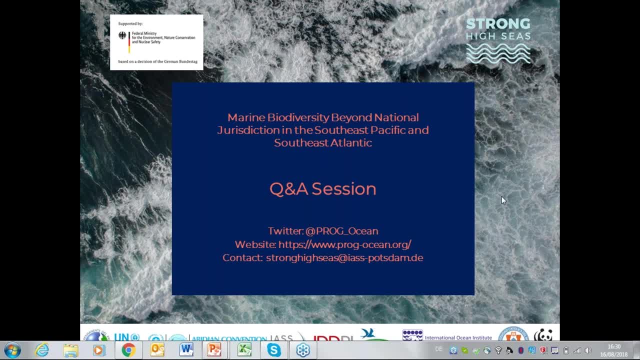 and ask you a question. So the question for you is: we have a participant that would like to know if, with climate change, it is already possible to see a trend in constant increase level of temperature in the South Pacific waters, as well as change in biodiversity distribution and occurrence of alien. 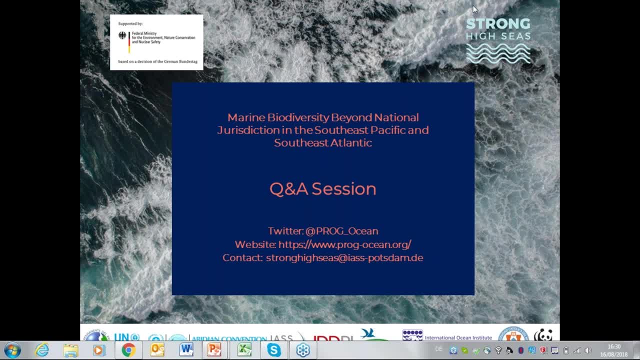 species. Yeah, so with climate change, what we are seeing is not only warming of the waters, but rather a trend to go to more that. the frequency of extreme temperatures, either high and low, is greater, So the impact on biodiversity is that it is harder for them to adapt to the 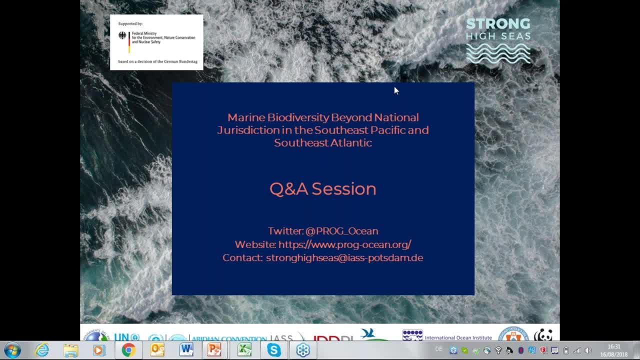 high frequency of this extreme temperature and also changes in salinity, because what is the climate change is driving also the very extreme precipitations along the coast, So the runoff is greater and the salinity changes are greater. So one of the threatens to the biodiversity of this region is 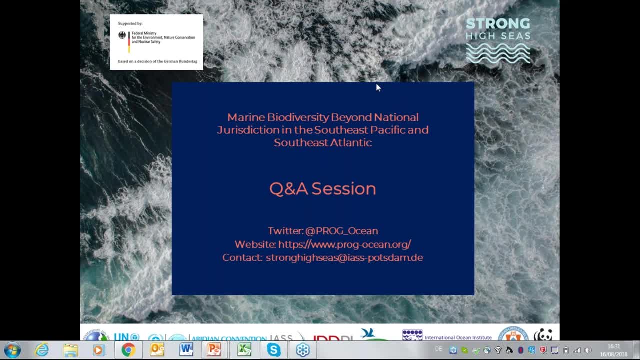 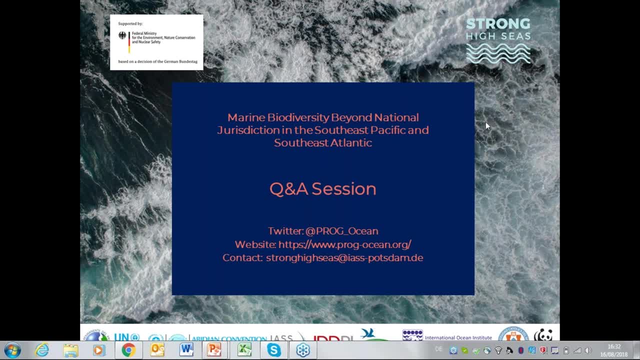 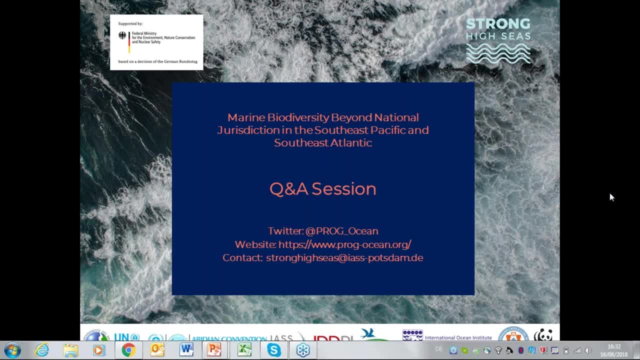 This is in regard to the oboes, And we have a question as to whether OBUS could become part of the BBNJ agreement in the future And do you think that this could possibly operate separately from potential clearinghouse mechanisms, or if OBUS could house all of the information associated with a future BBNJ agreement? 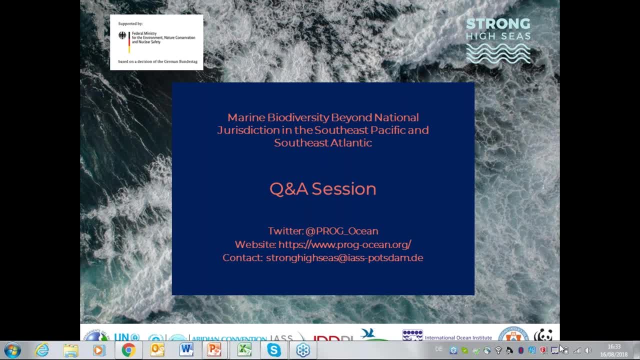 in regard to environmental impact assessments or the like, And I think Daniel is now unmuted too, so I'm not sure who wants to answer that question. I could start out and then see if Daniel has other comments as well. So my comments previously was that when we're thinking about new clearinghouses, 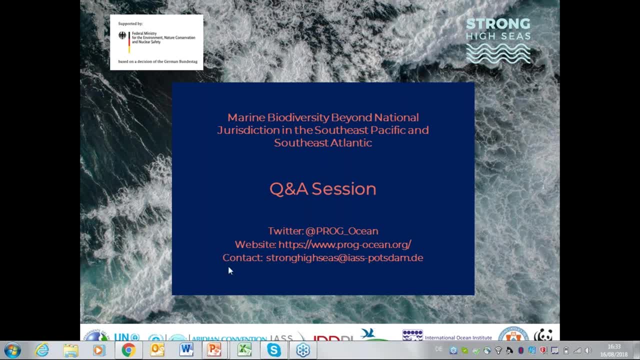 is to build on the existing infrastructure and OBUS is one of the pieces in that puzzle. So I feel that OBUS could play a very large role in providing biodiversity data globally for for areas beyond national jurisdiction. So I see that could be a very powerful role for OBUS. 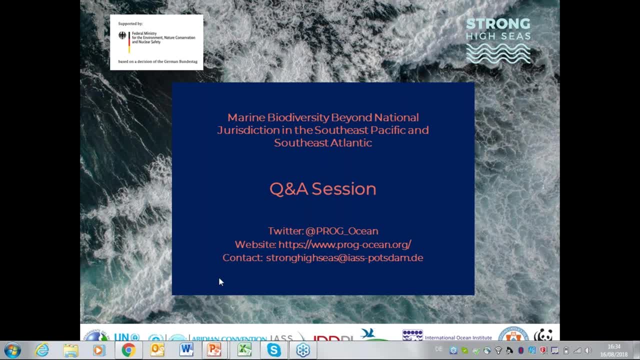 It wouldn't be exclusive. I think that there's many other types of data and information that need to be put together. My point was that there already are existing international institutions such as OBUS, GOOS, IMBON, and the list goes on, that these would be the building blocks that could be organized. 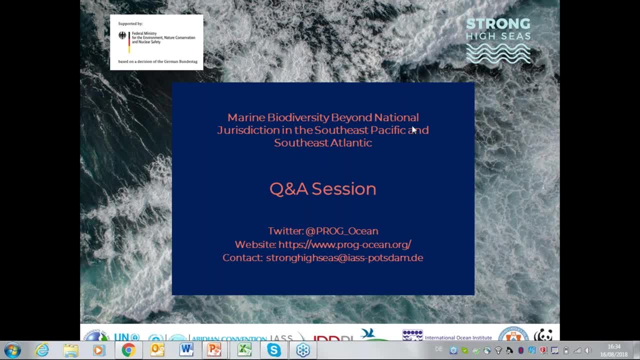 together to form what we might be considering the new clearinghouse. Daniel, do you have comments as well? Yeah, I think that's sort of the general direction that we've been heading with the thinking. I think one of the main questions right now isn't whether OBUS is going to be a critical 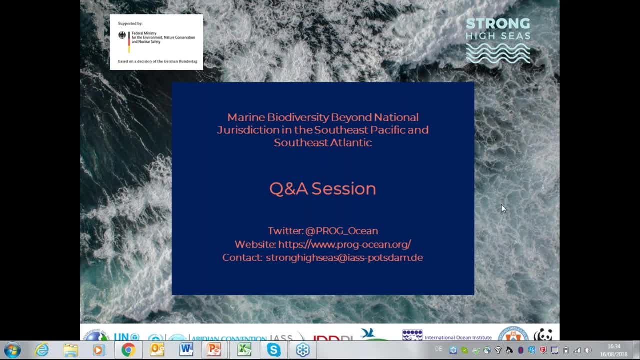 element. I think it's widely agreed, and has been brought up many times in the prep comms, that OBUS and the IOC in general are critical elements of any new agreement, And I think that OBUS will support a clearinghouse mechanism. I think the question is: 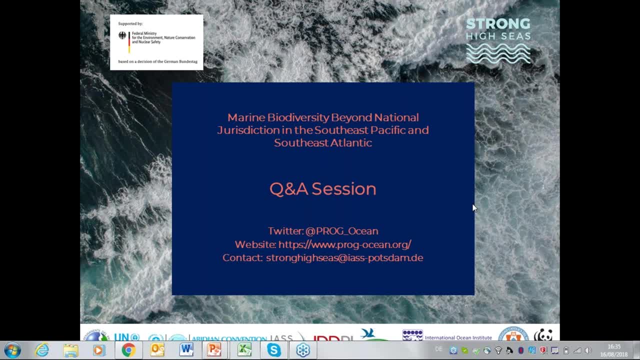 The broader question that still needs to be resolved is: what does that clearinghouse mechanism look like, How does it utilize the resources and support the resources that currently exist, And who are the main users of the clearinghouse mechanism? I think if we can get a little bit more clarity on that, it'll be a lot easier to answer questions. 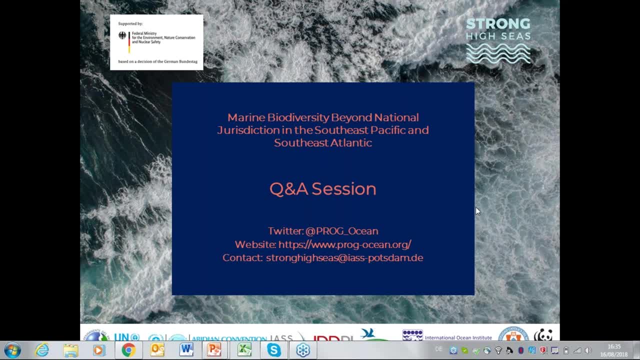 about OBUS's role. Yeah, Yeah, It's a little bit easier to answer questions about OBUS's role within it and how it would be used by policymakers and managers, But I think everybody is in agreement and there's been very little pushback at the prep. 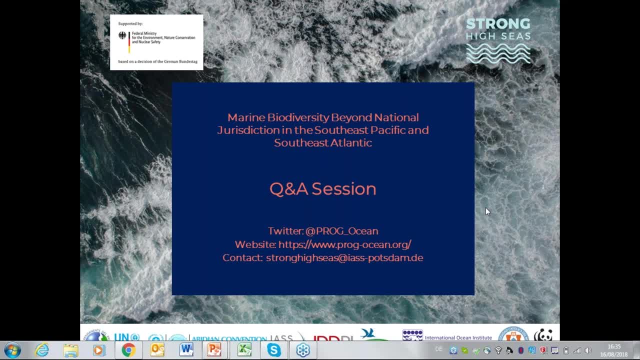 comms with respect to the role of OBUS as the major data warehouse for observations of marine species in BBNJ. Great, Thank you. Thank you, Okay, Thanks to both of you. Great answers. I think we have time for maybe one more question. 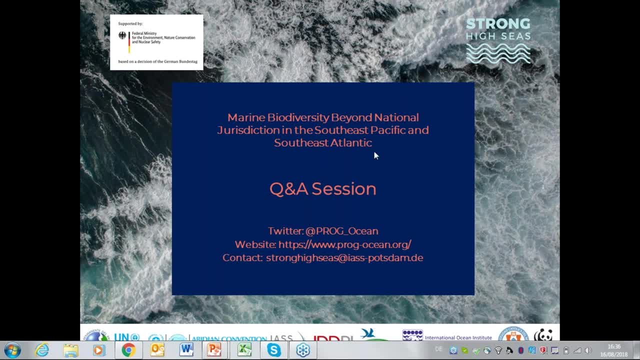 This one is for you, Ross, at BirdLife, And then we'll have to close the webinar for today. So the question is: what is the BirdLife international strategy to strengthen the current existing regional fisheries management organizations to address fishing issues in the high sea? 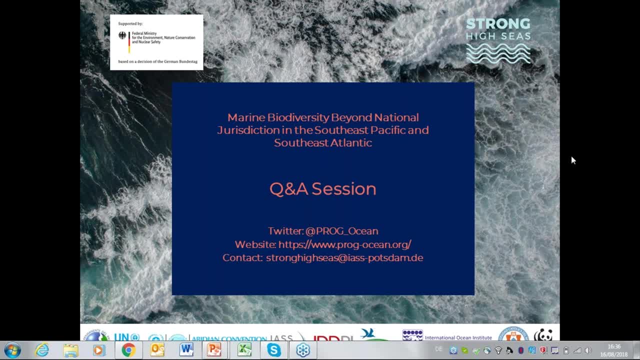 So Okay, Okay. So the first one is from Ross Yeah, So you're going to talk about- I don't know if you're interested there- Ross Yeah, So specifically around IUU, is that correct? That was the question. 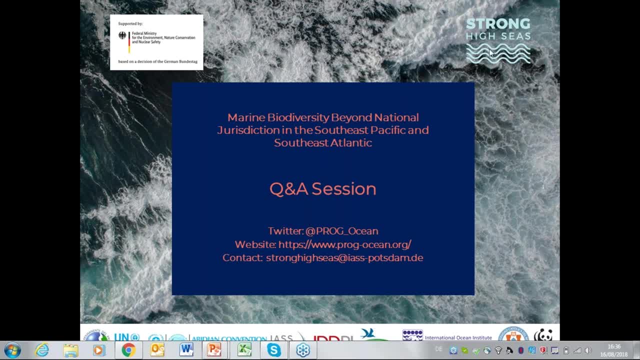 It's not No, It's asked in general. But if you have ideas in regard to IUU, I think that's Sure Okay. So yeah, in general, we're working incredibly hard- and have been since 2004- on engaging. 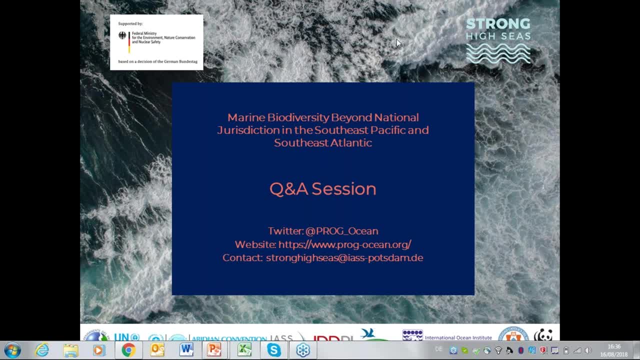 with RFMOs. The BirdLife strategy is not to throw bombs Right throw bombs, but is to get our hands dirty, knuckle down and do the work and work collaboratively with organizations. So we try to strengthen organizations. 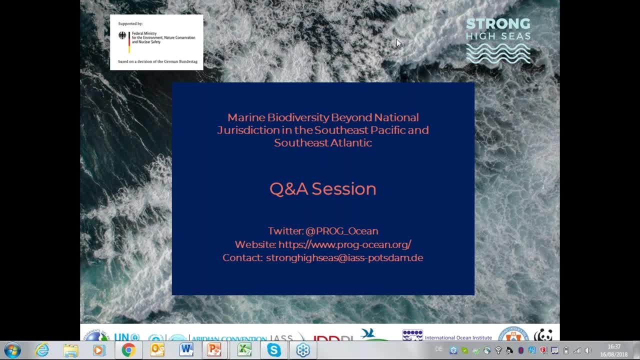 We try to understand where the challenges are and work to overcome those, and that approach has been really successful for our core interest, which is seabirds- getting seabird conservation measures approved, and we are moving more and more towards adapting that model into compliance and how to work with countries and with RFMOs to improve compliance. 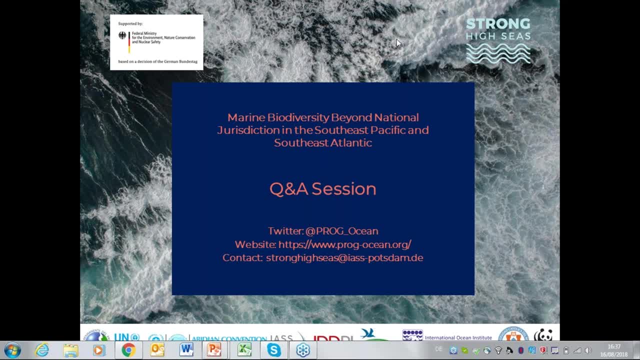 how to strengthen data collection systems, transparency, all of those things, And so our strategies involve exploring new technologies, like Global Fish Watch, and bringing those into the RFMO, understanding where we're working hand in glove with key fishing fleets. That's great. 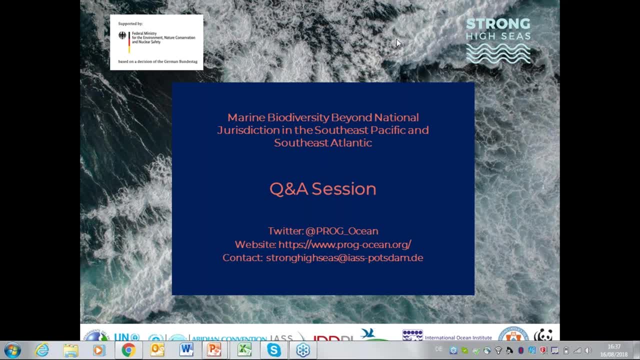 That have seabird bycatch concerns and trying to assist them in transitioning to become compliant, developing new systems and supporting other organizations, working collaboratively with organizations like Pew, Oceana, WWF and so forth to strengthen compliance systems. 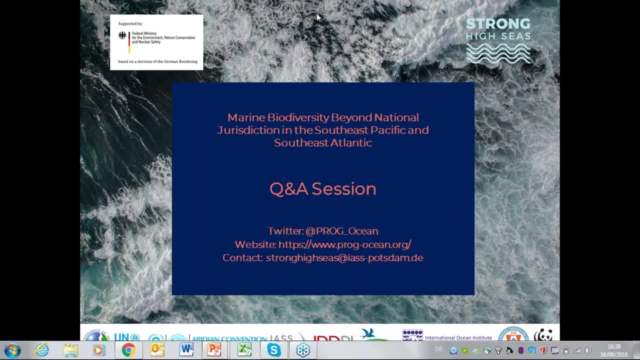 and observer programs in particular. So that's a fairly generic answer. I'm hoping it's sufficient. Okay, Great Thanks, Ross. I think that covers it. So I think that brings us to the end of our webinar for today. 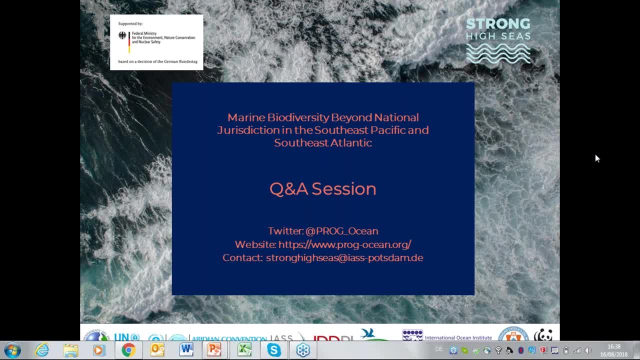 I want to thank all of the presenters for taking the time to come and give these interesting presentations and take a few minutes to answer questions afterwards. I hope all participants enjoyed the webinar. Thank you also for attending. Thank you, Thank you. 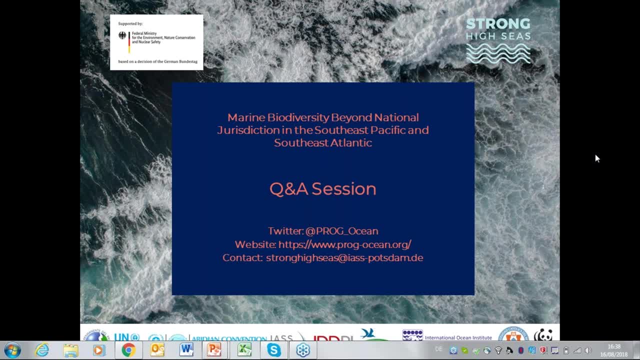 If you're interested in learning more about the project or have questions, please feel free to contact us at stronghisees at iss-podstemde, and we'll try to answer any emails or questions coming in as soon as we can, And also we will have the PowerPoint slides to share with participants, and then I also 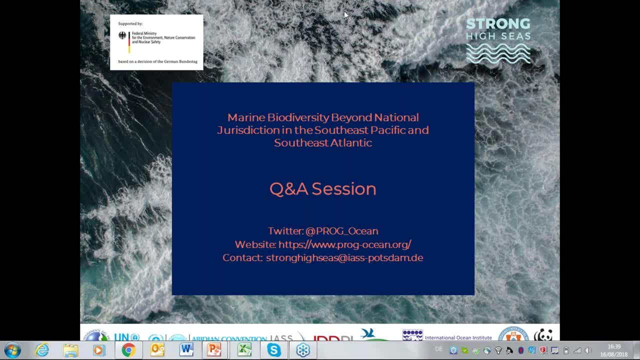 please encourage you to fill out the survey you will receive after the webinar. it's very short and would be very helpful for us. so with that, I wish you the very nice rest of your days, and thanks again. you, you, you, you, you, you, you.